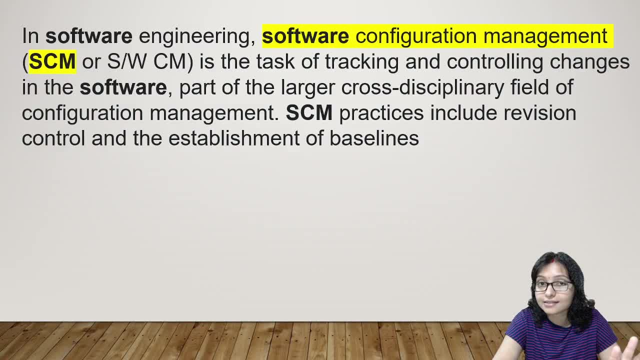 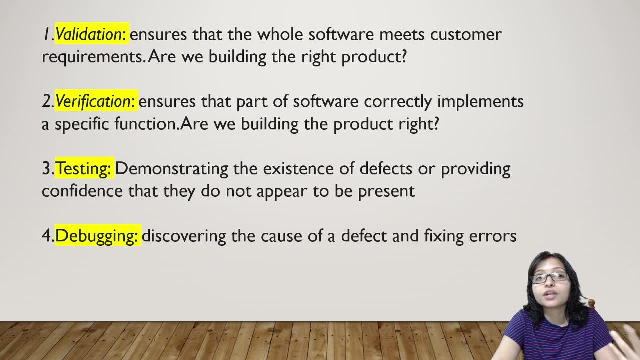 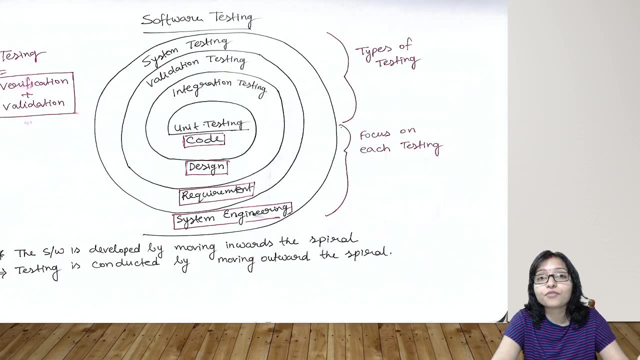 different types of coupling that time i am going to discuss. next one is: what is c scm? that is, software configuration management, how it is going on, what is verification, what is validation, what is testing, what is debugging after that? all types of testing, how it is going on, unit testing and 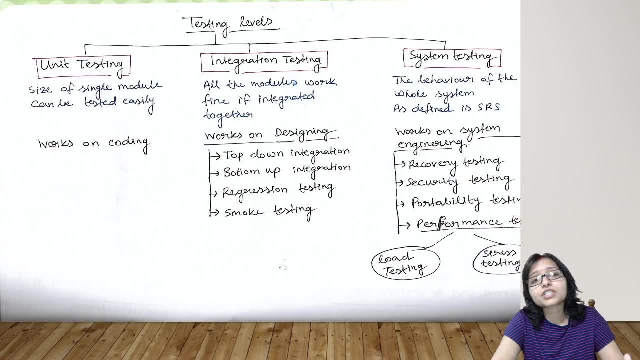 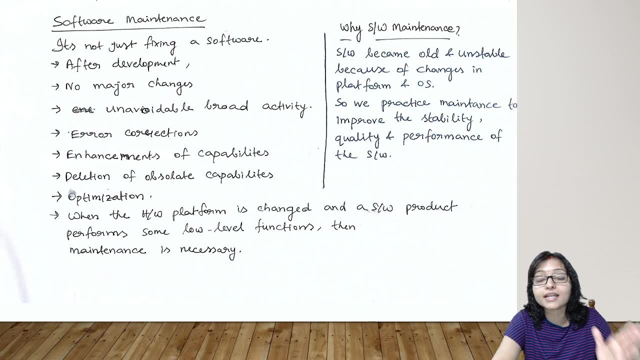 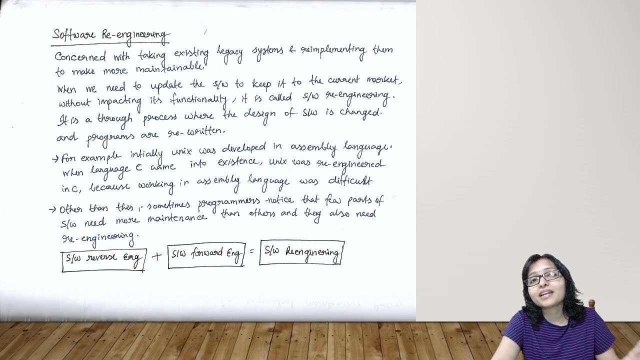 integration testing, system testing. what is verification, what is validation? everything we are going to discuss black box testing, white box testing, software maintenance, different types of maintenance- corrective, adaptive, perfective, preventive- each and every type of maintenance. i am going to discuss re-engineering and reverse engineering. what? 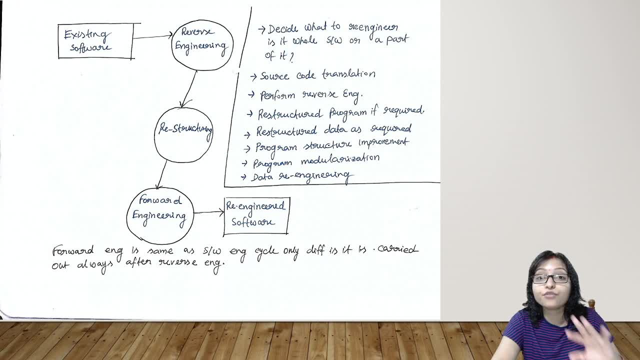 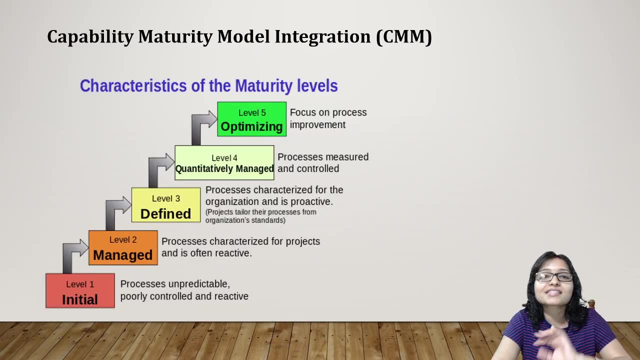 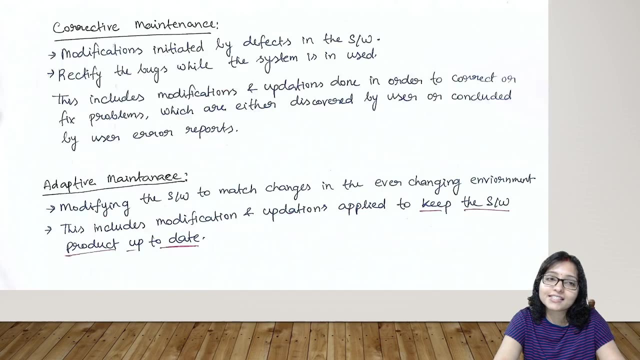 is the difference between re-engineering and reverse engineering. i will discuss clearly and you can see all are my handwritten notes here. after that we will discuss the cmm level also and finally i will end the video here. so now you can understand so many topics i am going to. 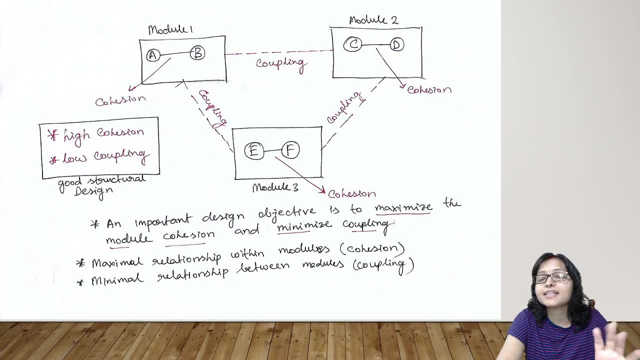 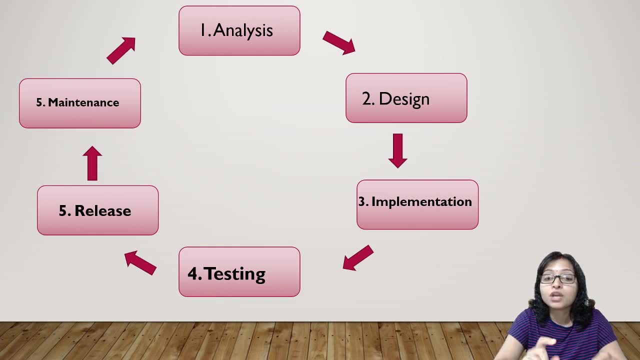 cover in this video. so please watch this video till the end and definitely subscribe to the channel. click the bell icon to get all the latest update and notification. don't skip it, don't pause it. you have to understand each and every point clearly. then only you can attempt the question. 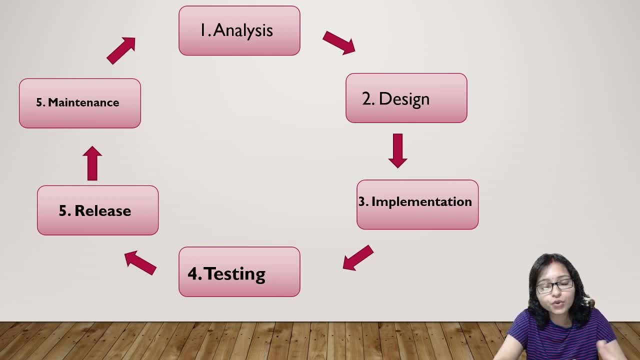 and i will suggest you try to play this video repetitively multiple times so that, like a story, you can remember software engineering. it is my guarantee that if you will watch this video and watch this video till the end, then you will understand what is re-engineering and reverse engineering. 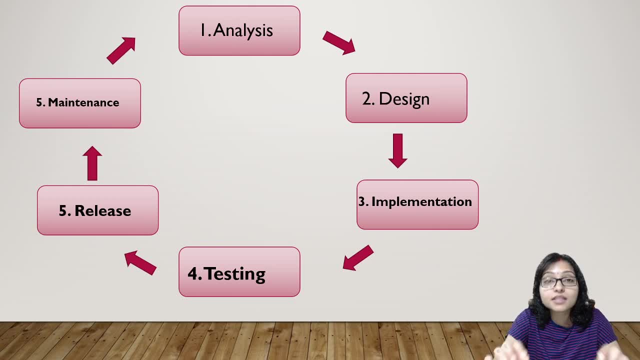 at least four to five times. if you will listen this video like a story also when you are doing other work, then also you will be very much confident about each and every topic because ultimately you are learning with someone who have five years industry experience and two years teaching experience with ujc net qualification. so now start it in the software. 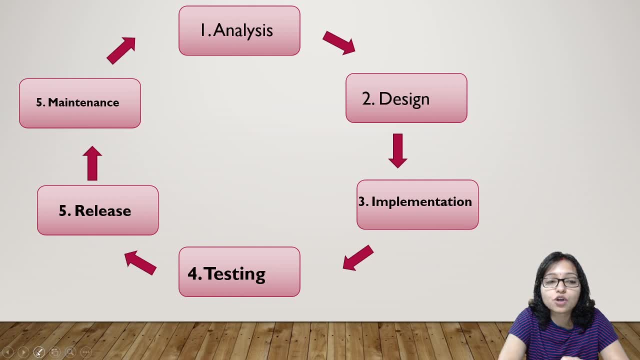 engineering. what are the phases first of all, why we are learning software engineering and what are the parts are there? when you can do the mind mapping, then it is very easy to understand and then it is very easy to remember. so first part is analysis. analysis means it is the requirement. 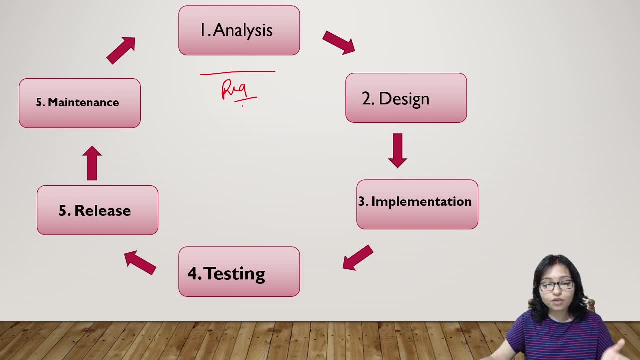 analysis: what is the requirement? it can be the requirement of: what are the specifications, what are the features customer is asking. so that are the features, what I am going to do. next analysis can be that how many team members are required, like how many developers are required, how many database engineers are required, how many 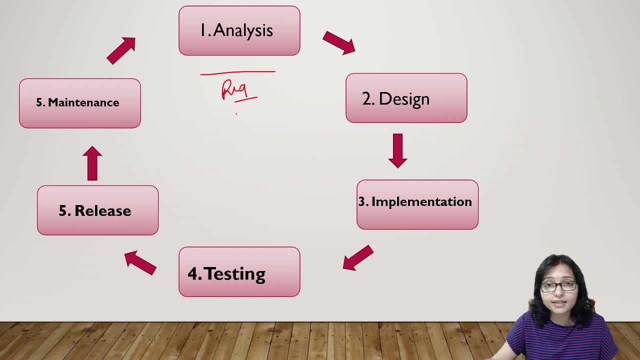 designers are required. that is also analysis. and after that the time analysis: what is the total time? that is also required. then the cost analysis: what will be the cost? so these are the very important analysis in the analysis phase. after that we are coming to the design phase in the 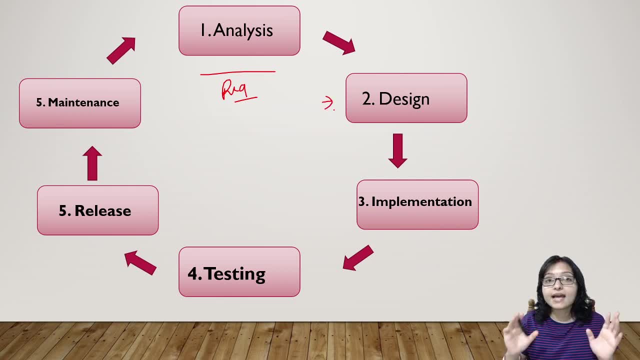 design phase what we are going, because design is very important. whenever you are trying to build a house, then designing is a very important part: how? what will be my planning of the house? so, in the same way, whenever you are trying to develop a software, then software design is also. 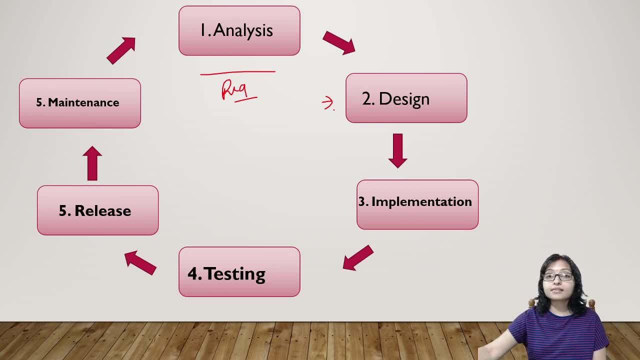 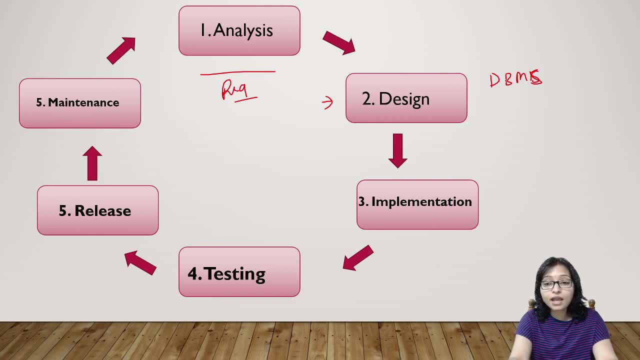 activity diagram, sequence diagram and ear diagram also there. this all the diagram we are doing so that how it will actually work after designing. now your designing part is done, after design we are going to come to the implementation means ultimately, now coder is coding it, but it is a very 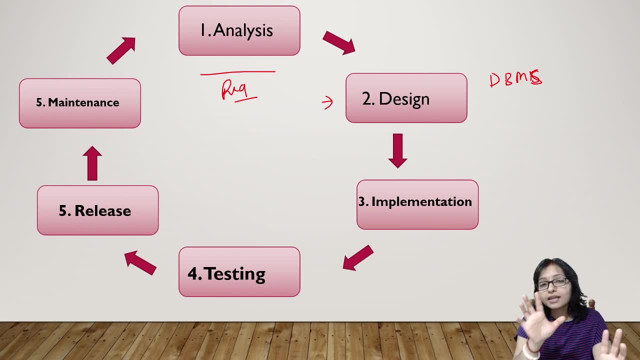 less time comparatively to the very total life cycle of a project implementation part is a very less time. after the implementation it is coming to the tester team. so remember one thing: implementation is doing by the coder and when coder is checking that the program is running successfully or not, that is called the debugging. that is a very important concept most of the time. 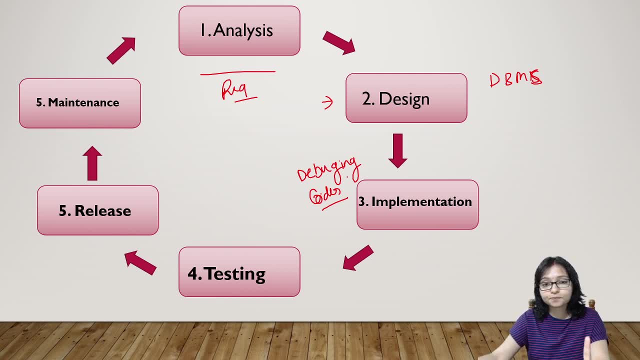 students are getting confused with debugging and testing. so debugging means when you are writing a code and you are checking it that it is working correctly and after that again you are fixing it. that is doing by the coder. that is called the debugging, and whenever it is coming to the tester. 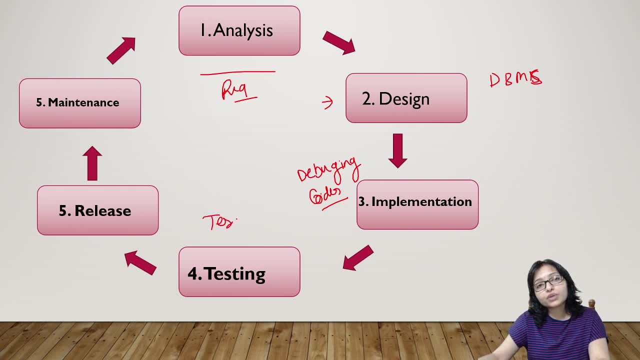 so tester don't know, maybe it is coming to the tester and then they are doing the debugging and maybe tester don't know how it is coded. so tester is testing that that the functionalities are working fine or not. so there are two types of main testing, that is, black box testing and white box. 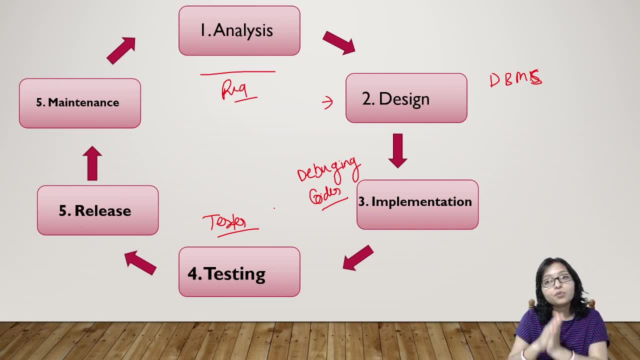 testing. in the black box testing, they are providing the input and they are getting the output. is the output is correct, fine or not? in the white box testing, they are testing through the code. okay, so we will learn all that. all types of testing don't. but next comes theる pizza paris. that is all right, and then i'll talk more about the review gap. 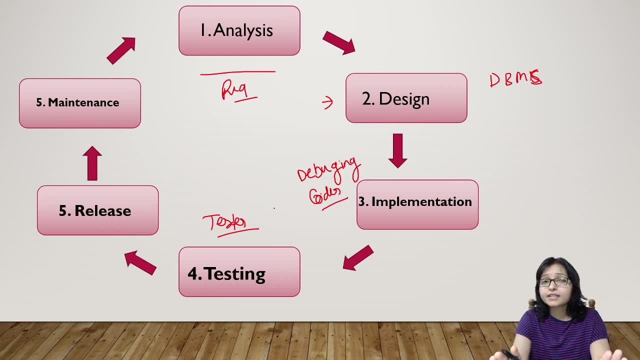 wow. so this is very interesting, right, it's quite positioning, just like that. so these are the 我们 decay��� қ43ные. thats cool. now the next bit is about the how do we find out that we do this? how did we还有 mustache? you can see here. this isid somewhat similar to the first part gone, but i want use thatag in going out, so i'll just go ahead and i'll share at point spray and come back again. be back one moment. i'll start talking, so please understand how to do so. after doing everything you have, now your project is work. now your something. part of the version is 2 to 1, so now you are sending it to the client means it is for the release. so after releasing, may not? that is 70 percent of the project. life cycle is the maintenance part and it is the most ast injustice. the maintenance piece is the réalité that it is not going to happen forever. 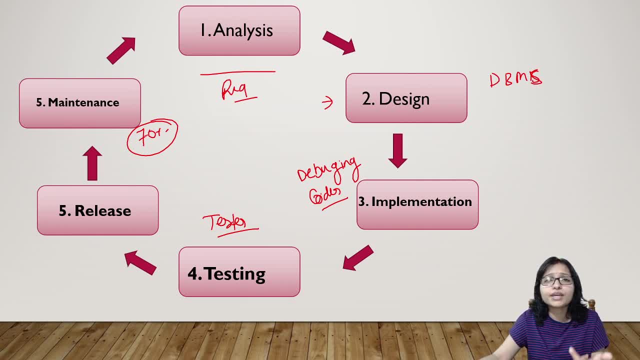 companies, because ultimately, maybe one year, two year, you are developing a project, but after developing when it is running in original environment, then the maintenance part is very important. so then we are doing the maintenance part at the time of maintenance part. there are different types of maintenance: adaptive maintenance, corrective maintenance, perfective. 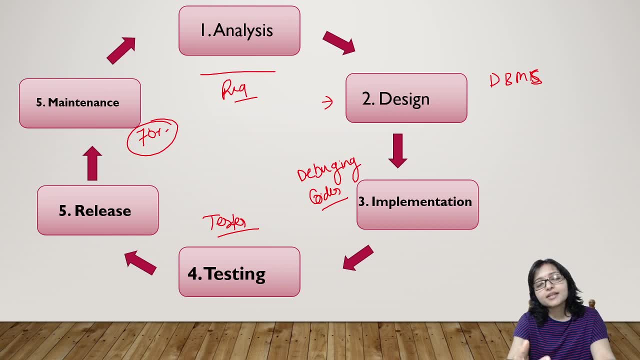 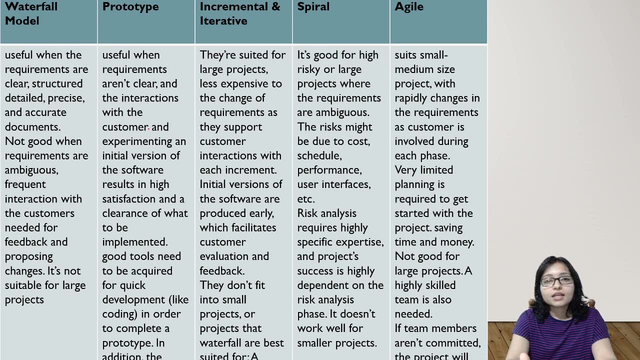 maintenance, preventive maintenance. what are those maintenance that we will learn. so now come to the next part, that is when you are developing that, as per the project criteria, different types of models are there. what type of project you are going to build in that situation you will take? 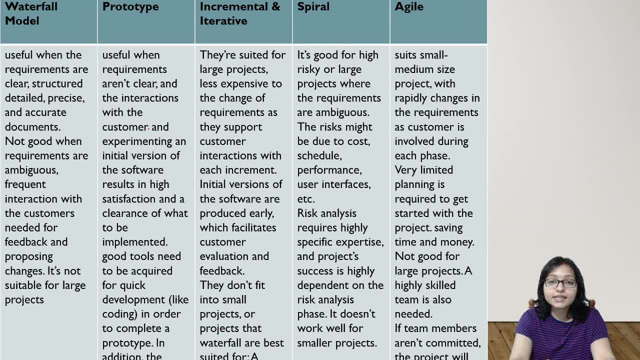 the decision. yes, i can go for the model. this models are telling you if you are following this model, then it will be easy to implement your software. so there are mainly a focus on the question coming: waterfall model, prototype model, incremental and iterative model, spiral model and nowadays it is very popular. that is agile model, so waterfall model means it is very. 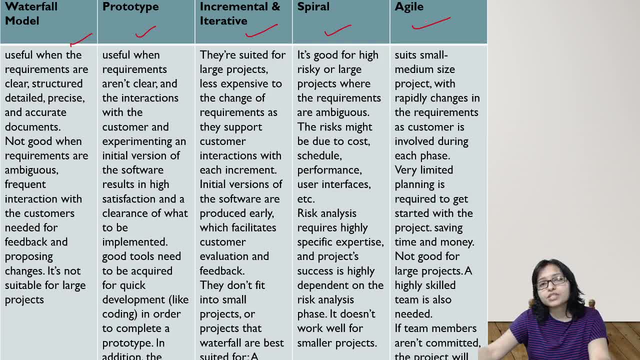 very easy and very small, very small project, like when- nowadays no companies are using that, but when you are doing a school project, small project, are going for the waterfall model, mainly how the waterfall model working. it is just like a waterfall. what is telling by the waterfall of? before ending one phase, here you see the different types of 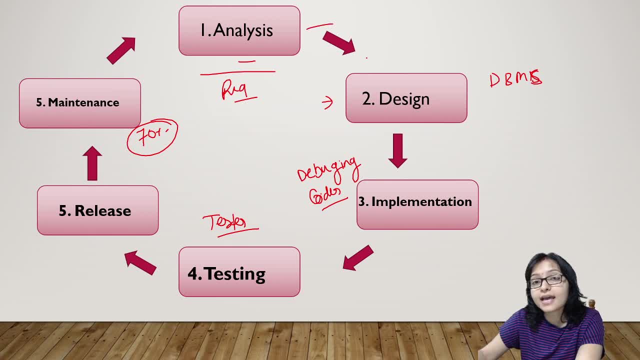 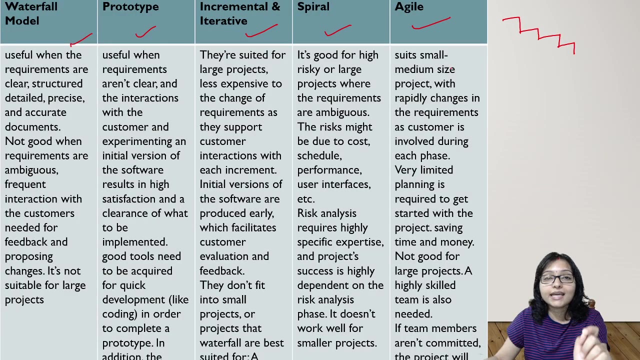 phases right. so before ending analysis, i cannot start design. before ending design, i cannot start implementation. before ending implementation i cannot start testing. that's why this is called a waterfall model. before ending of a project, before ending of a part, you cannot start the next part. that's why this is called the waterfall model and you cannot back also that. back that if. 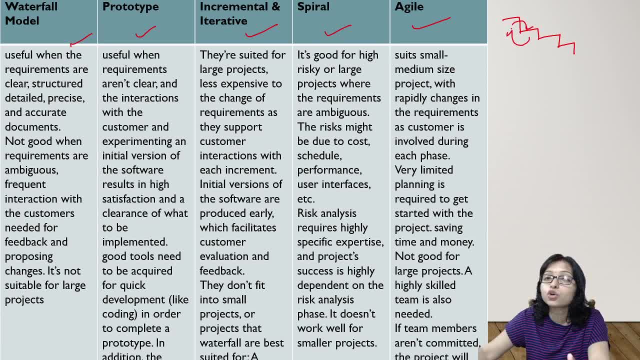 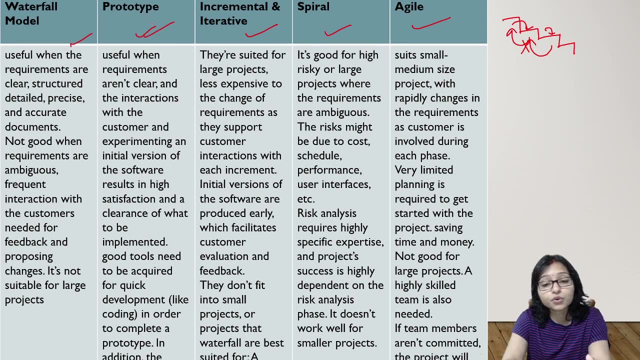 you have already started the design part, then you cannot go to the implementation part. if you have already started the development part, then you cannot go to the design again. okay, next one is the prototype. when we are using prototype model. prototype model is using when customer is not able to explain you what type of project he want- means the requirement is not clear to us. 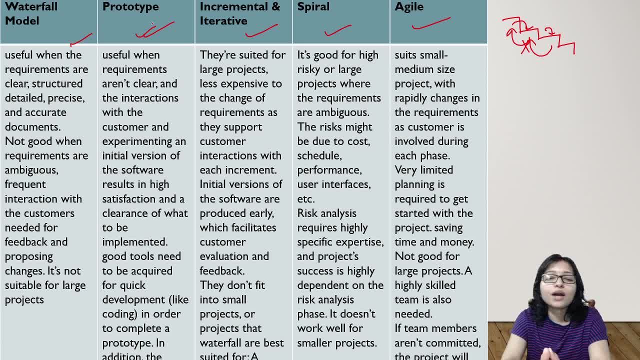 like that one. anyone is telling you i want to make a house, but he is not able to explain you how the house will looks like then the, then the engineers are showing them that there are different types of of model of the house, maybe from the images or some models, then from the model he is choosing. 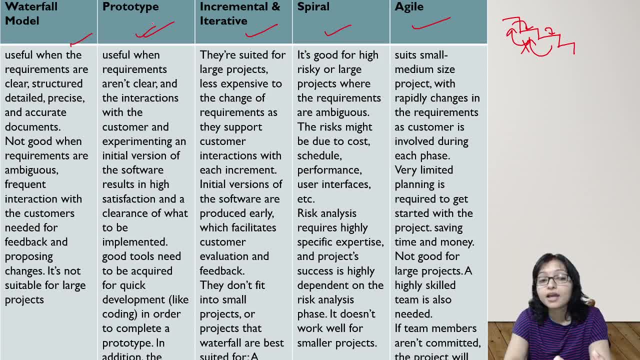 yes, this design is very good, so I will go for this design and after that maybe with that design, as per his purpose, he is doing some changes. this is called the prototype model, so for the software also, when customer is not able to explain what type of project he wants to build, then software 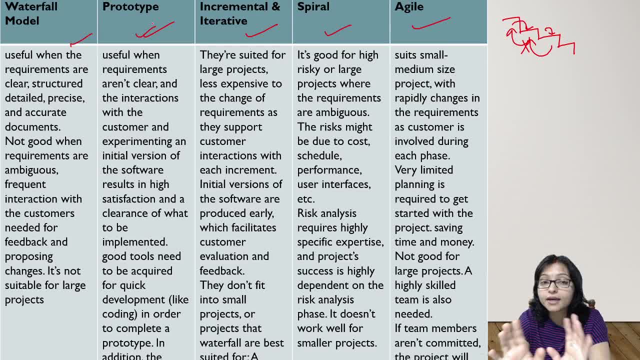 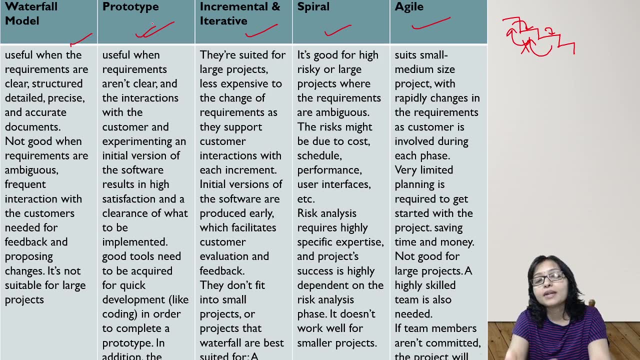 developer are showing a dummy. it is not complete version. they are showing a dummy and by watching the dummy now, customer is able to understand, customer can able to explain it. yes, this is my exact purpose. then we are started building the project. that's why it is called the prototype. 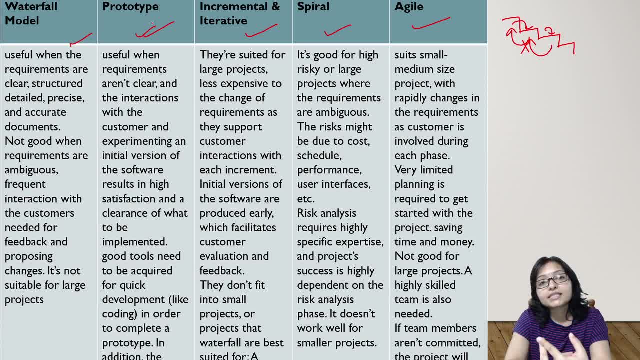 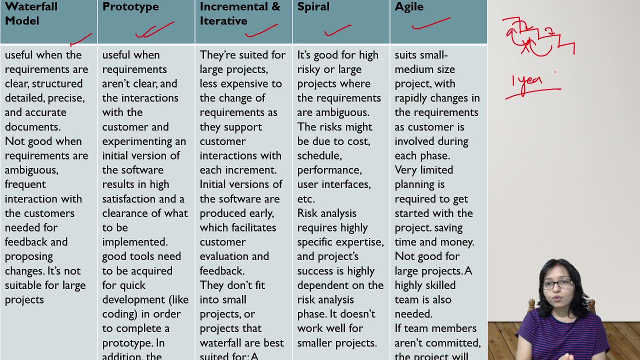 next one is incremental and iterative. so incremental and iterative means what? maybe you project is a big project, maybe it will take one year. so it is not possible that i will start now and after one year i will release to the customer. it is very risky because maybe, if there is any, 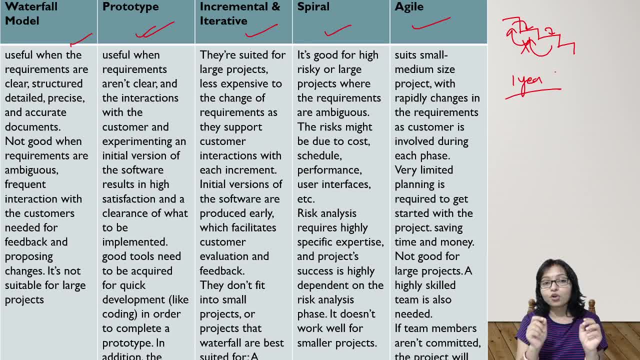 problem in understanding the project. if there is any problem in requirement gathering, then it can be a blunder that maybe customer told you that, yes, i want a bicycle and you make a motorcycle. after that customer told you: no, my purpose was bicycle, you made a motorcycle, i am. 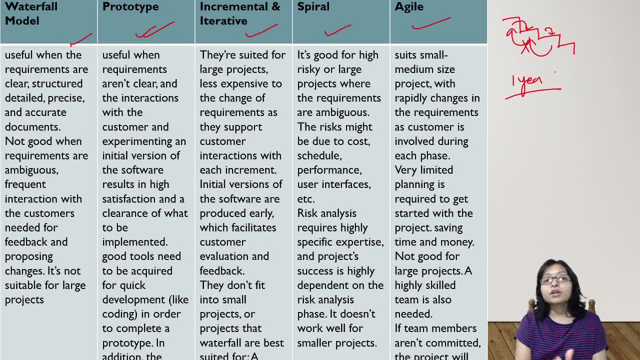 not going to take that, so it will be a blunder. so that's why companies are going for the incremental and iterative model, because when they are doing the incremental model or the iterative model, then they are dividing the project into small, small part. maybe there is a total project. 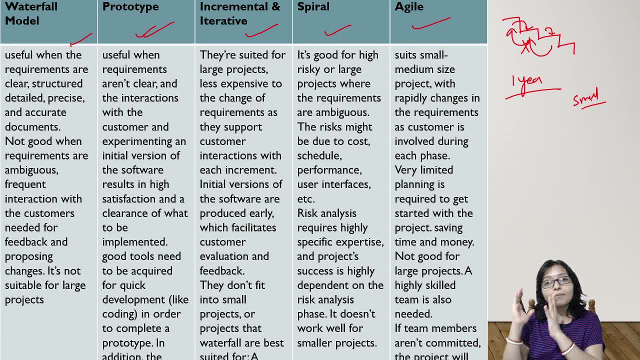 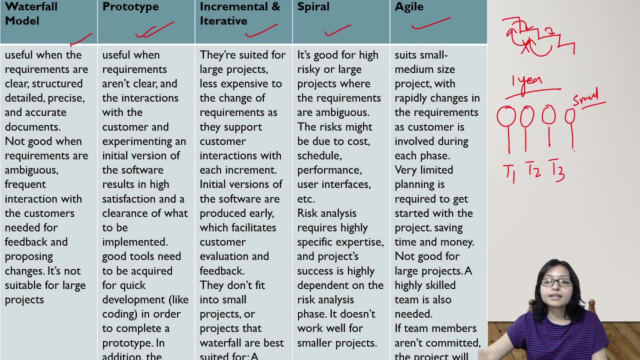 they are dividing some module wise or some month wise time wise. module wise means when it is parallely, they are dividing the project. this part will be done by the team one, this part will be done by the team two, this part will be done by the team three and this part will be done by the team. 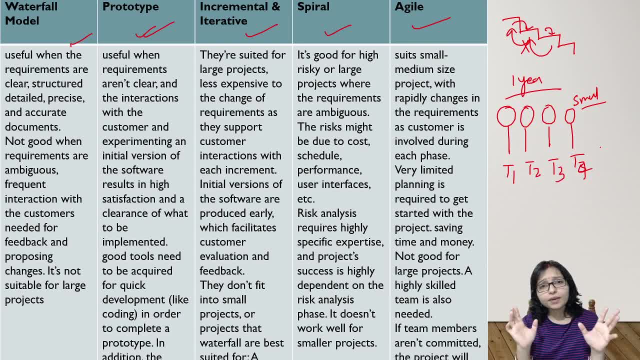 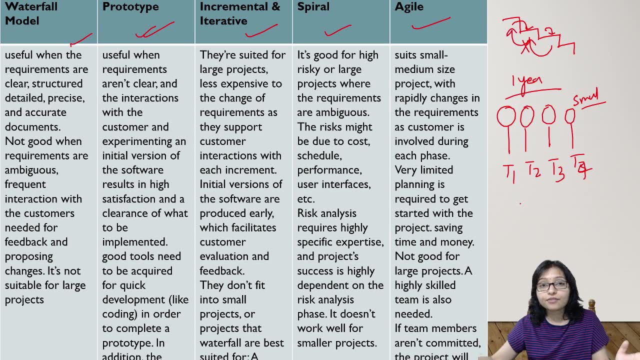 four and everyone is doing parallely and whatever feature is done, it will deliver to the customer, be like that key or total team is working together and some part of the project. it is a big feature. the project is dividing into some small, small parts. so one feature i will develop that is: 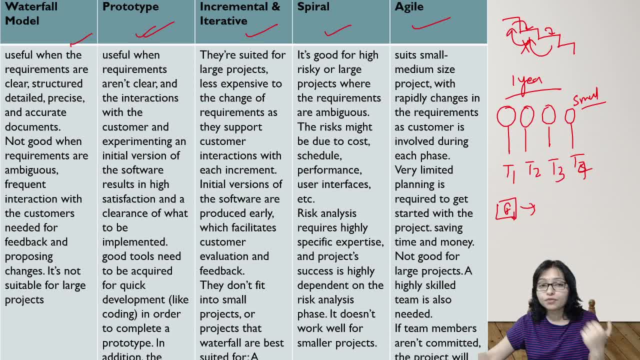 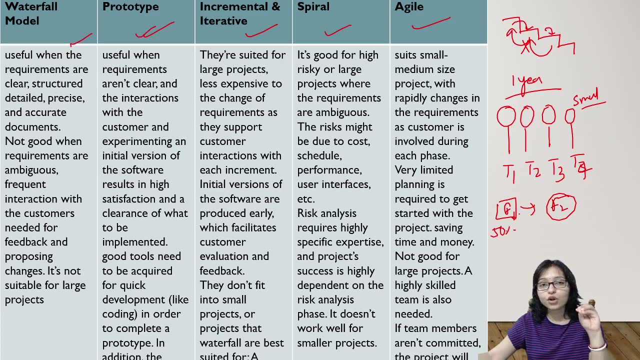 feature one. it will be sent to the customer. customer feedback will be taken- yes, it is correct or not? then we will go for the next feature. or it can be also possible that one feature is taking more time. so 50 of the feature. we will do, the basic model we will do, and after: 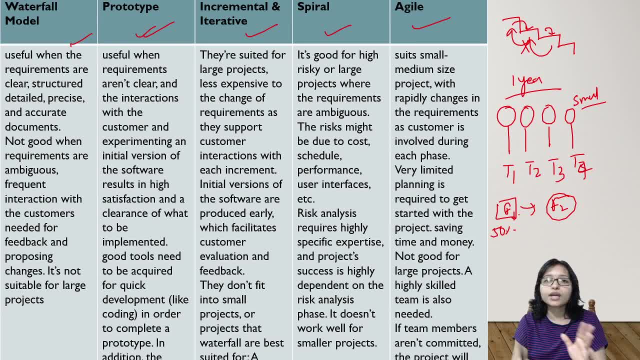 that we will send to the customer. customer will tell: yes, this is okay. now i want to add this, or maybe i want to change this, so then we will do the remaining 50. this is the main concept of incremental or the iterative model. there is the difference between increment and iterative, so 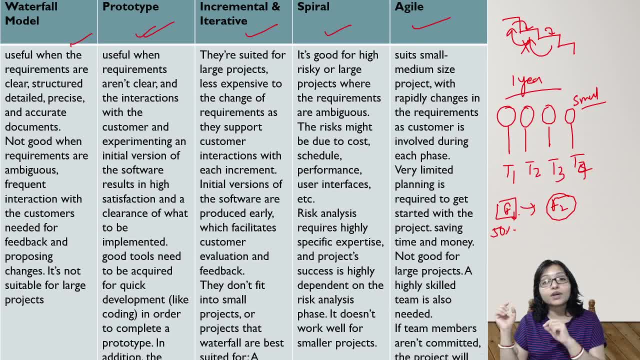 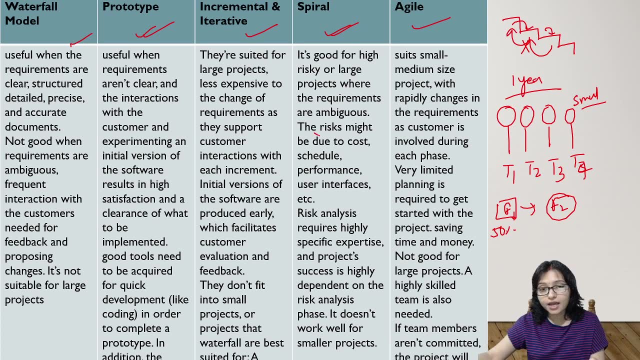 if you are interested then i will upload the video. what is the main difference between incremental and iterative? so let me know in the comment section. next one is spiral. so spiral is main focus of the spiral is the risk management. here the main focus is the risk management. in other model risk management, risk analysis was not there in every phases. 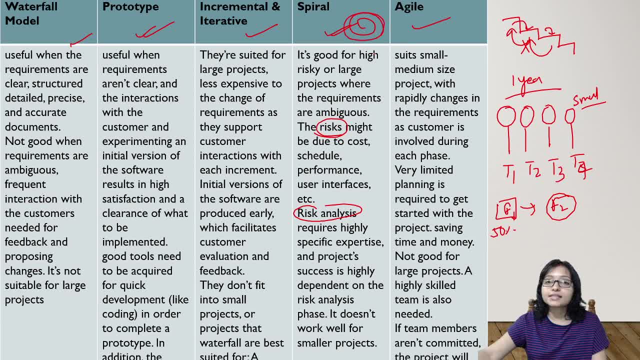 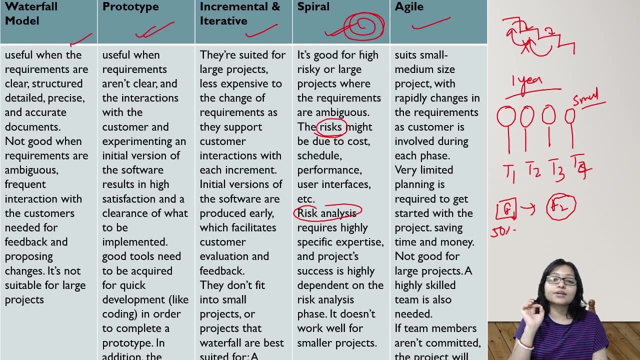 it is look going like a spiral, one by one, phases, incrementally. it is going on. but the new feature is added here, that is risk analysis. it is not done in other model till now, so that is the main advantage of the spiral model. remember that, the risk analysis. next one is the. 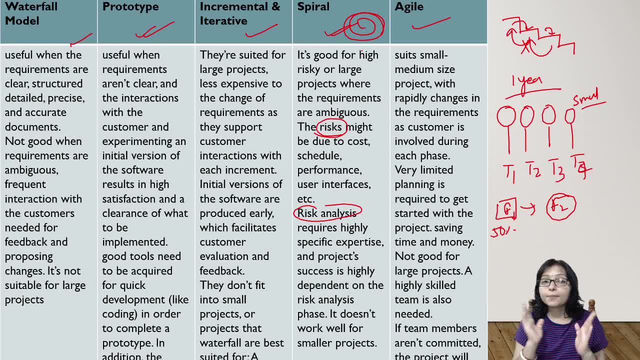 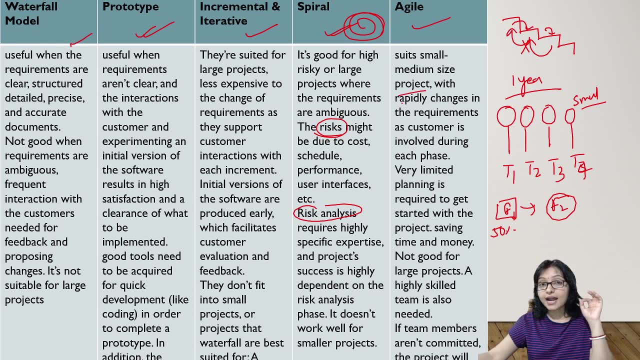 agile. so what is agile as i is the combination of iterative and incremental model and the main focus of the agile is the part of the main focus: the small, medium size project it is doing and the rapid change is the main focus. the rapid change it is customer can do anytime, any changes. 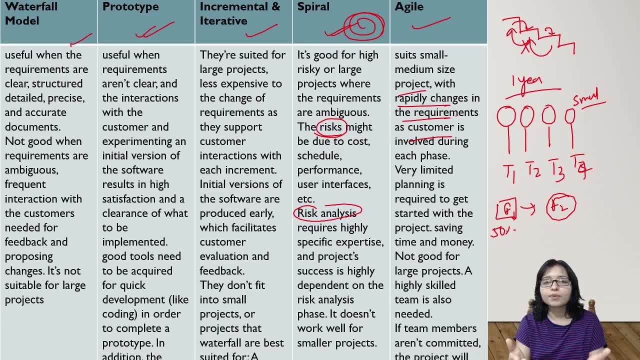 maybe you have done something for last one month. then customer is asking: no, i want to change there. so you have to be that much flexible. that much flexibility is required so that anytime any changes can be done, and that's why your project structure, your coding structure, should be. 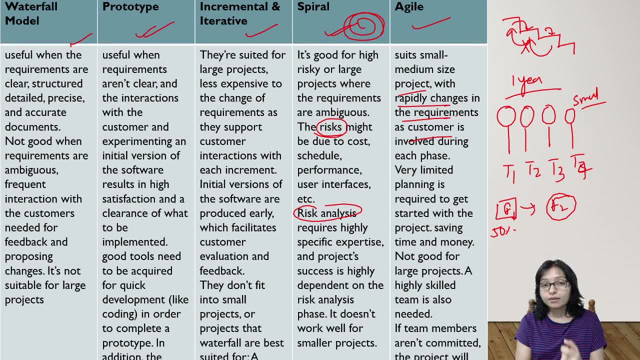 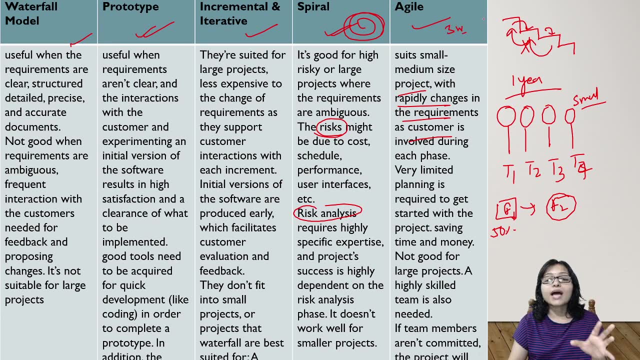 efficient. all the team members should be also very much efficient and each and every project with dividing in a sprint and each and every sprint will be maximum three weeks, maximum, right. so that is the main feature of the agile and in my channel i am giving you the link in the: 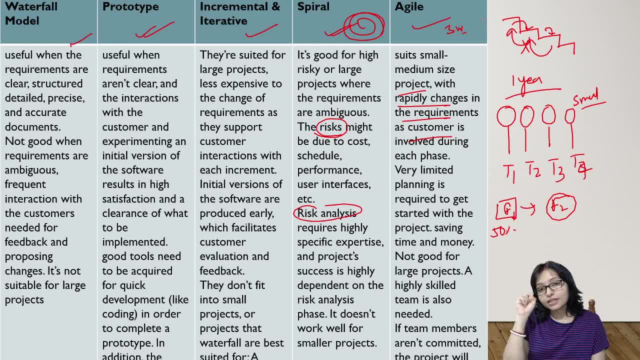 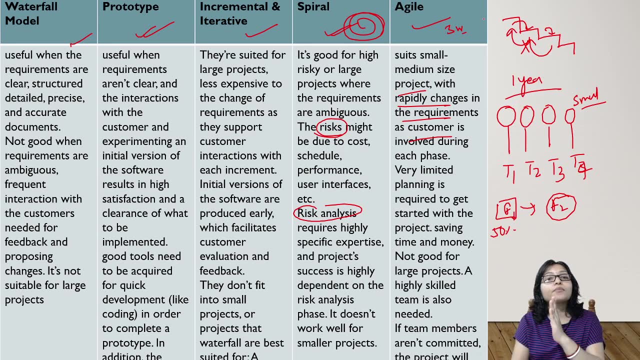 top for the agile methodology- detailed discussion is also there- and for our all other sdlc model also detailed, detailed discussion i have already done. you can watch the recording. so this is the total analysis of waterfall, prototype, incremental spiral and agile and it is your quick revision chart also. 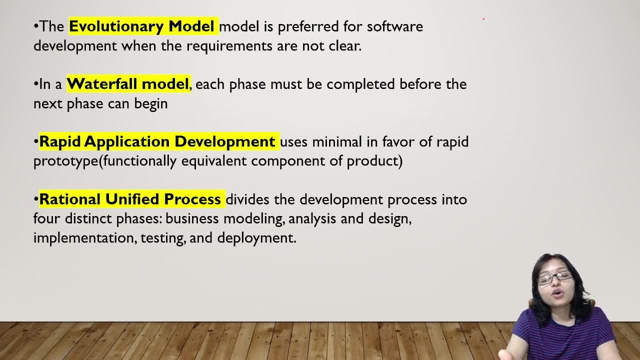 next one is: evolutionary model is also a type of prototype model only. okay, this is a type of prototype model only don't be confused with the evolutionary model. it is a part of prototype model and we are using it, not clear waterfall model, that is. we already discussed rapid application model. that is red red we are using when there is minimal flavor of 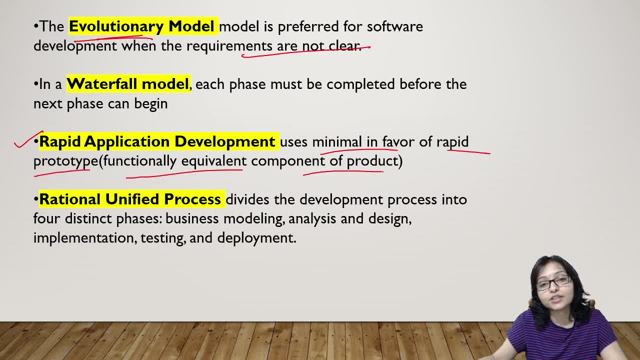 rapid prototype functionally equivalent component of the product. so maybe some product you have done data that is functionally equivalent. then we are going for the rad and rational unified process that is dividing the development process into four distinct phases. it is dividing into four distinct phases, that is business model analysis. 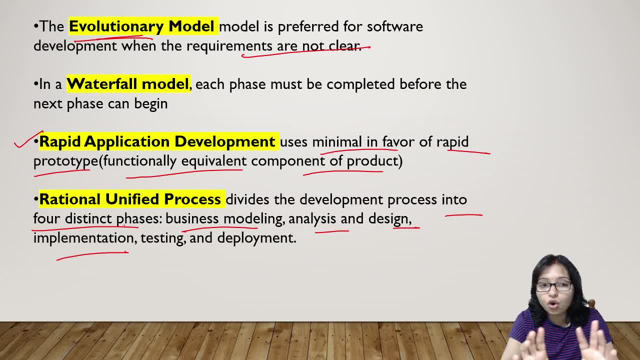 design and implementation. so these are all the models from where question are coming. if detail analysis is required, you can refer to my videos of detailed analysis. and what are the videos are not available, let me know in the comment section. i will upload that video and i will see you in the 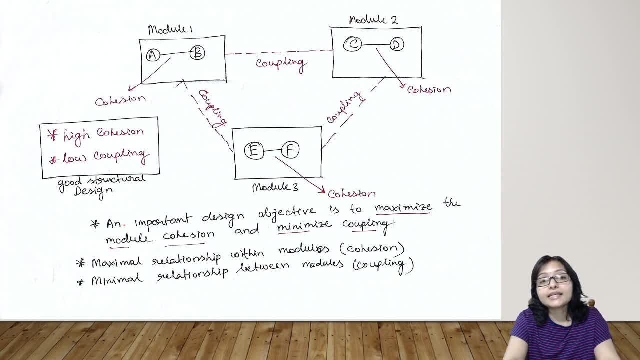 next videos in detail. now come to the design. so in the design part, when you are doing the design, then you have to your in your mind- it is very carefully. you have to handle that- that when i am dividing the project it is a total project. right, the total project is a big project now in my team. 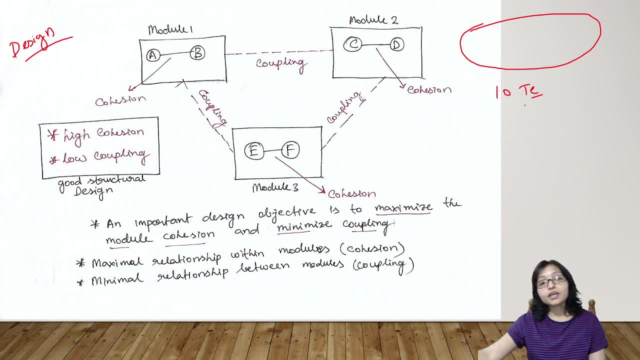 there is 10 team member. okay, so i will divide the total project into four distinct phases and i will divide the total project into 10 parts so that i can give the responsibility- i can share the responsibility to each and every team member. now, whenever you are sharing the responsibility to each, 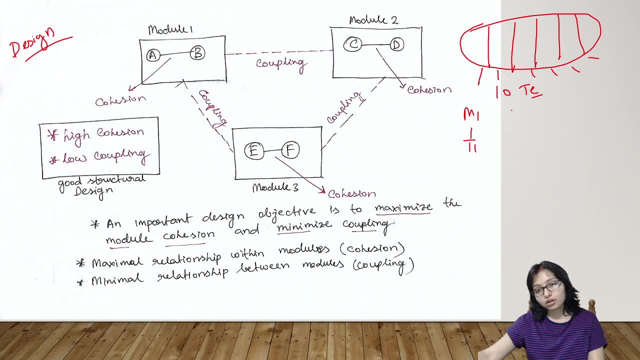 statement: team member: module one for team member one. module two for team member two. module three for team member three. in that way then, it should be like that keep between the module two and the modules- like module one will be not that much dependent on module two or module three- between. 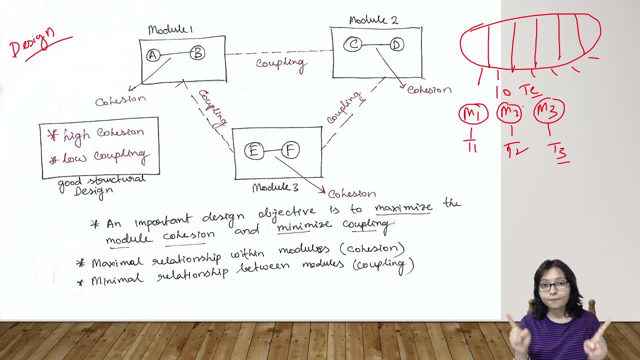 the module. there should not be that much dependency like you and your neighbor. that much dependency should not be there. rather than more important is how much you are related with your family member, how much bonding is there with your own family member. that is more important, right? so that? 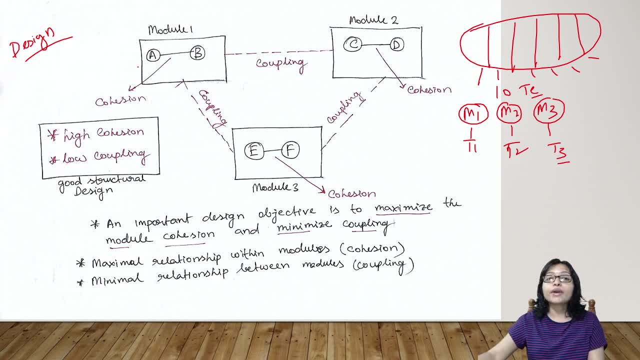 is why cohesion. what is cohesion? cohesion means inside the module. what are the features? are very much related. that all the features together you will take in one module and what are the features are different. there is no relation. you will separate it into the other module and at the 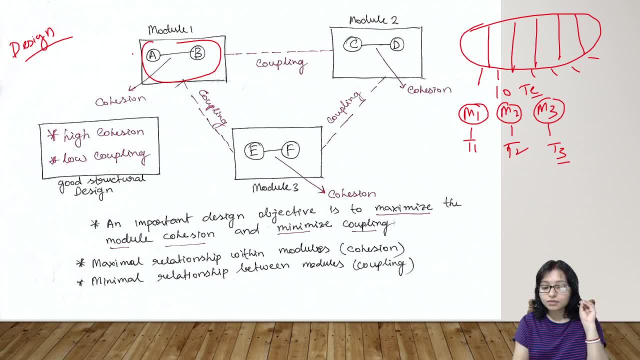 time of dividing the module. you have to. it is. it is very important to keep in your mind. that's why we are telling this is the over, which is the over, which is the focus point. that is why we are telling that high cohesion means inside the model. inside in a model, the elements should be very much 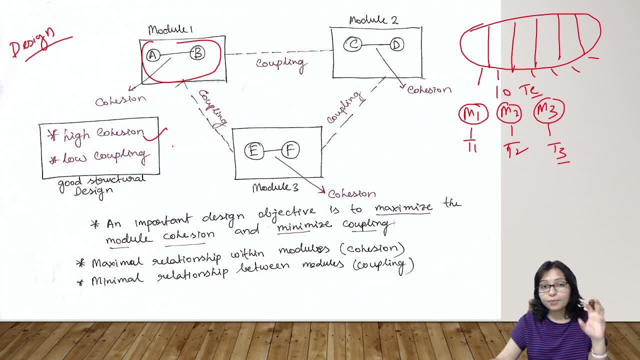 related. the bonding is very much important, but one model to another model, one module to another module, coupling should be. low means it is not possible that there is no dependency, because some dependency will be there as ultimately you are going to be integrate all the module and it. 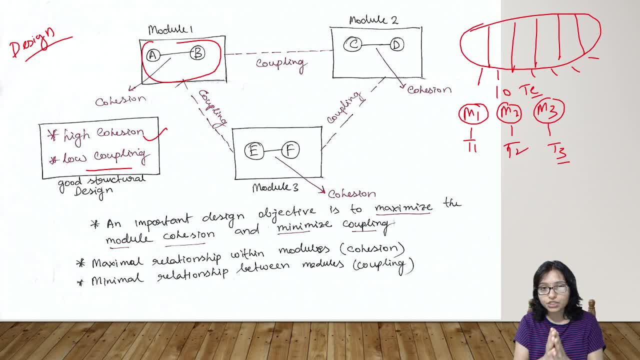 is a total sequence and ultimately it is going to be a project. that's why it is not possible that there will be no relation. there will be some relation that we cannot avoid, but as much as possible, try to lose it. try to lose it. that's why we are telling high cohesion and low coupling. 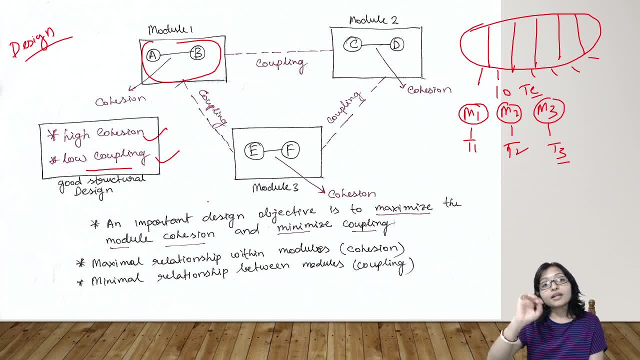 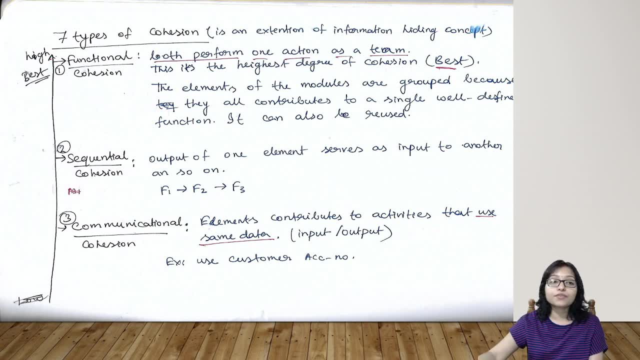 now we are going to do the different types of cohesion and different types of coupling, and this higher to lower is very important. which one is best and which one is worst. so seven types of cohesions are there: functional cohesion, sequential cohesion. functional cohesion is the best. that is number one. next one is sequential, next one is communicational. 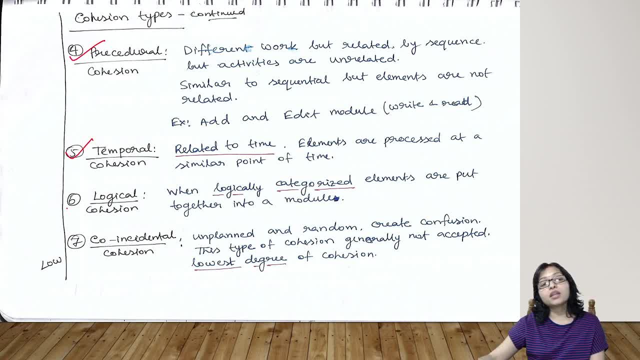 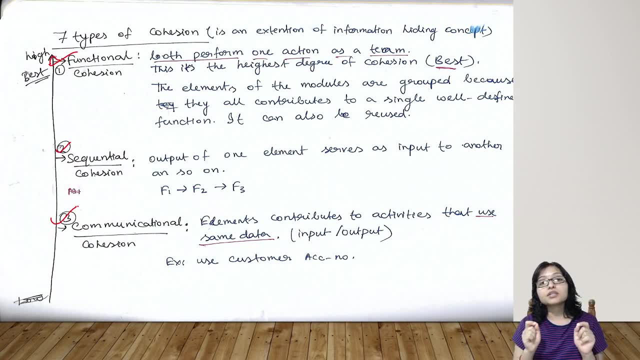 next one is procedural, temporal, logical and coincidental. so first of all, functional. functional means: what is that that? see that i have already marked the main line. both perform one action as a team means when the all the some element, like i am taking example like registration and login. registration and login are very much related, right when you will register in. 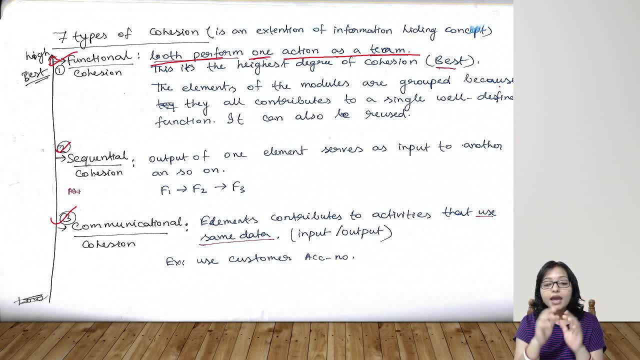 your website, then after that only you have to log in and all the data of the register is: ultimately you are using that username and password for the login. so registration and login is very much related. so that's why maybe you can combine these two feature together. that is called the functional. both perform one action as a team. this is functional functionally. 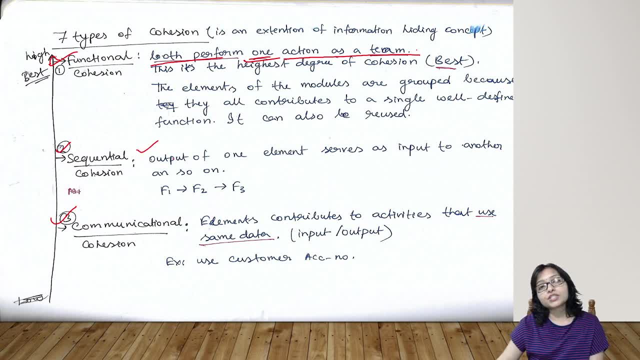 they are related. next one is sequential. sequential means what that output of the one serves as a input to another and so on. so sequential. so you are trying to purchase a product, so you will add to cart. so add to cart is a feature. after that you are trying to payment. 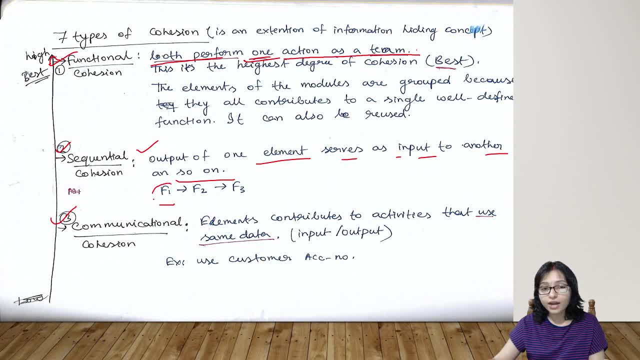 so, after add to cart, what are the product you had to cart? that is a element. and then, finally, that is only sending that. these are the is placed. now the payment is required. so now it is going to the payment. so it is a sequence right. so act to cut, after that you have to do the payment. this is 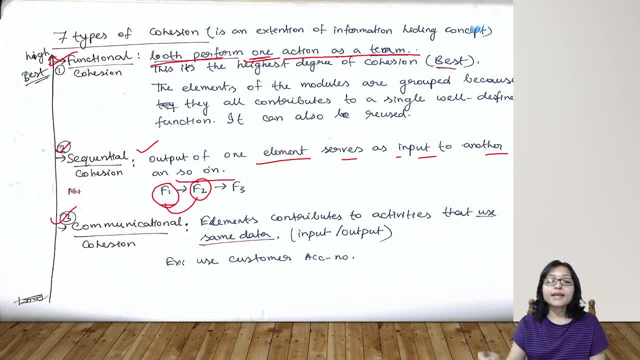 a sequence. they are related sequentially. next one is communicational cohesion, communication. communication means say that the it's contributes the activities that they use the same data. same data may be account number. account number is the same data. so account number of a customer is used by everyone, used by 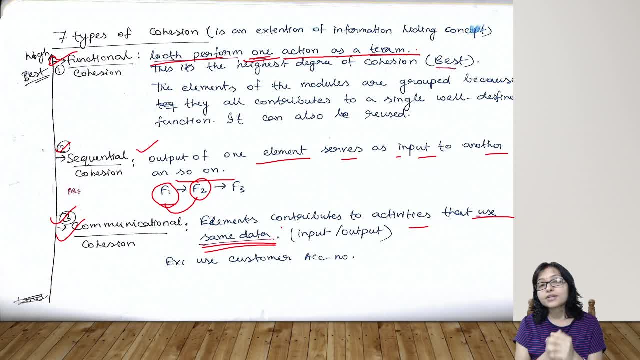 everyone, but mainly when any customer is trying to withdraw money. so money withdrawal or maybe, and he want to add some money in the account. so these are to other distinct functionality. but withdraw and add money that are using same account number. that's why they are related. they are using different features. so many functions can be used for the same account number. so next one is: 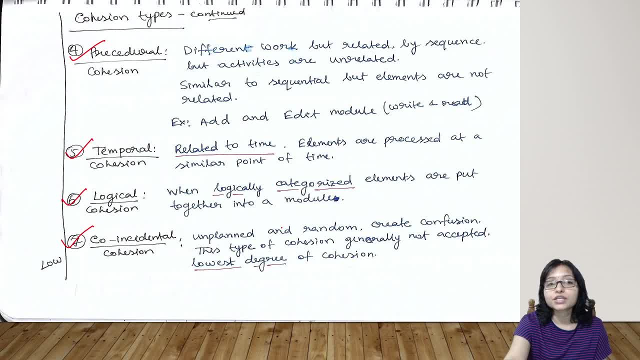 so they are using same account number. so they are related, they are using using the same data. that is called the communicational cohesion. next one is the procedural cohesion. procedural cohesion is that different work, but related by sequence. but activities are unrelated. here. very important here. this is very important: student are getting confused with the 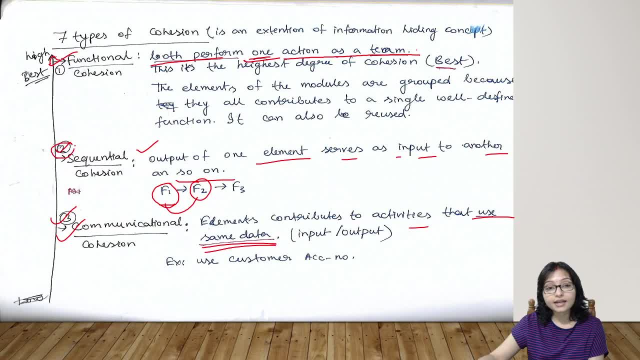 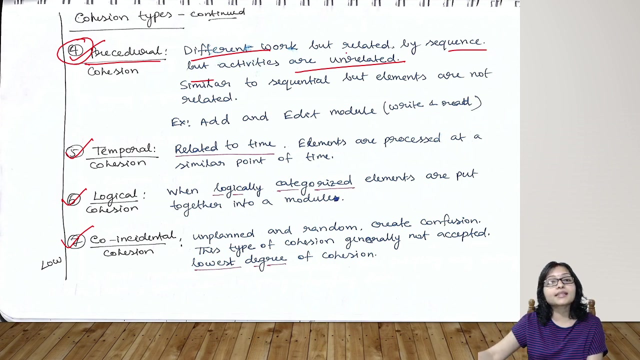 procedural and sequential. see that here it was one element, input and output. see that one element serves as input to another. i will add to cut. then this will be the input in the payment. that was the sequence. that's why it was the number two. but here this is not that much good, because here they are. 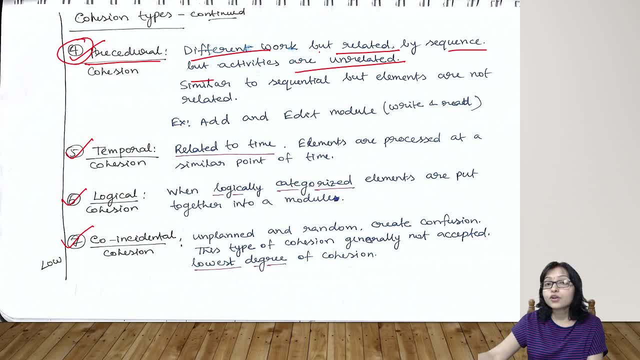 not related. they are the different work. they are not related, but they are related as a sequence, how that add and edit functionality, read or write functionality, someone is added, someone add something. maybe I add my profile, maybe I add my profile image. after that I am editing the profile image. so these are totally different two things, but they are related as 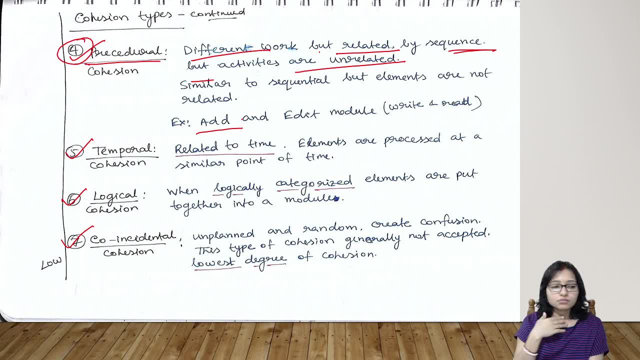 for the sequence. I am uploading now this image and I will upload- I will edit that image- another image. so these two images are different totally and these two functionalities are different totally. no need to combine together, but still we are combining. that is called the procedural. next one is the temporal. temporal is related to time. this is not at all good. that same time you 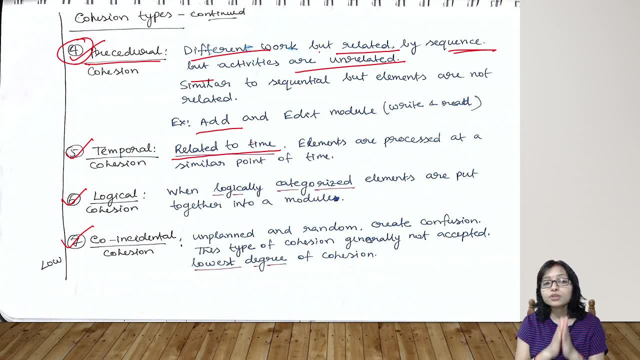 are doing the work. that's why you are combining in one module. that is not at all good. so they are related to time only. there is no functionality relation. there is no input relation, output relation, no sequence relations. still you are putting in one cup, one module for as there is timely related. that's why temporal is not that much good. they 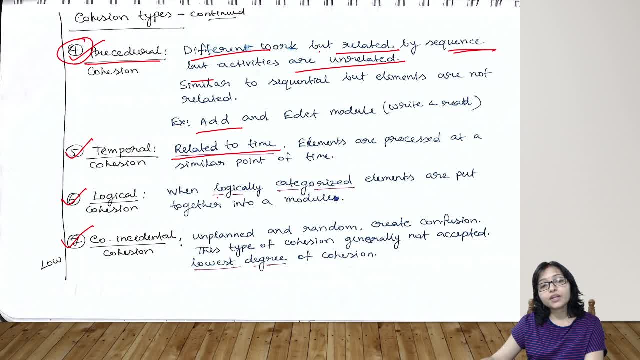 are related to the time. logical is when logically categorized. when it is logically categorized, you are categorizing like. the same logic are there as per your coding. when you are doing the coding, as there are, same logic is there as per your coding. so this is why temporal is not that much good. 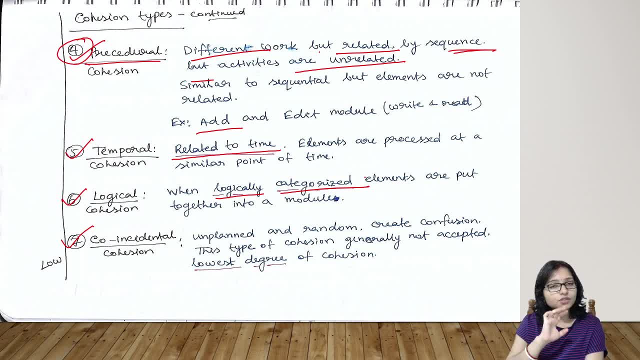 using. that's why you are putting in same module. that is not at all good. and last one is the coincidential. actually there is nothing. actually there is no relation, nothing. coincidentally, randomly, you are putting: it is totally unplanned. it is totally unplanned or randomly you are. 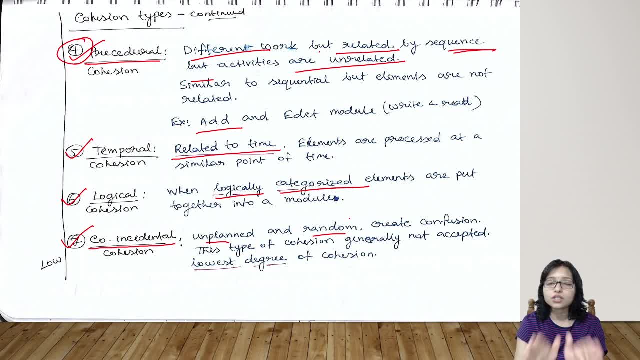 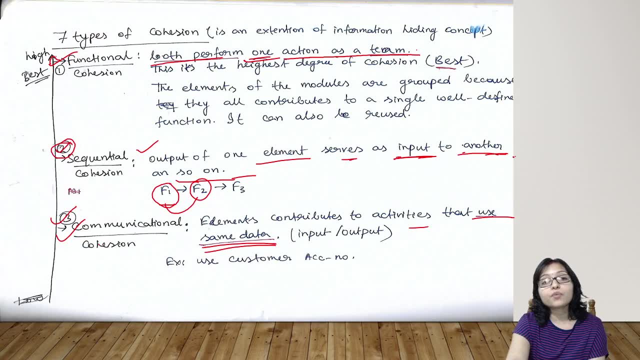 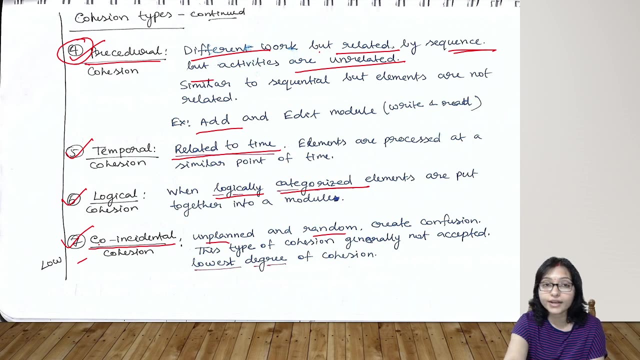 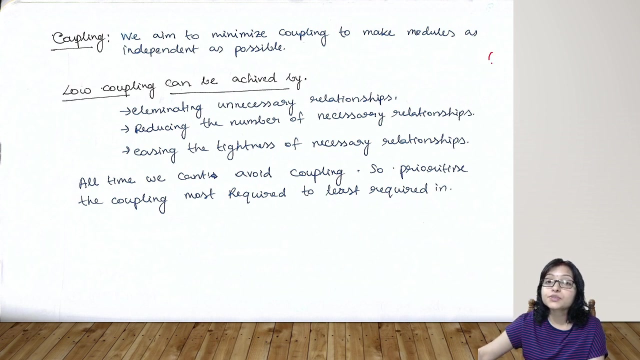 putting some functionalities in same module. that's why it is the worst one. so coincidential is the worst one. that's why remember the sequence. first one was functional: sequential, communicational, procedural, temporal, logical and coincidential. this sequence is very important. next one is coupling. coupling means between two module, between two module. this is module one. 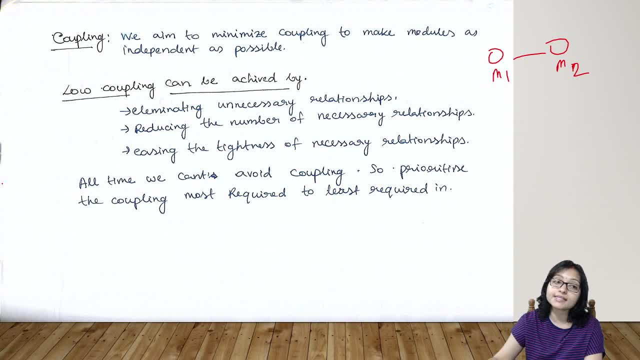 this is module two. till now we was using that in a same module. when you are adding the limits now, what will be the relation between two module? so here, eliminating unnecessary relationship, you have to eliminate, reducing the number of necessary relationship. if there is necessary relationship, then also, as much as possible, reduce it. and erasing, easing- erasing, not easing means. 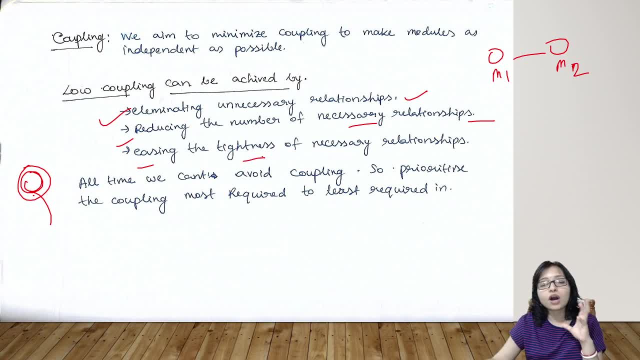 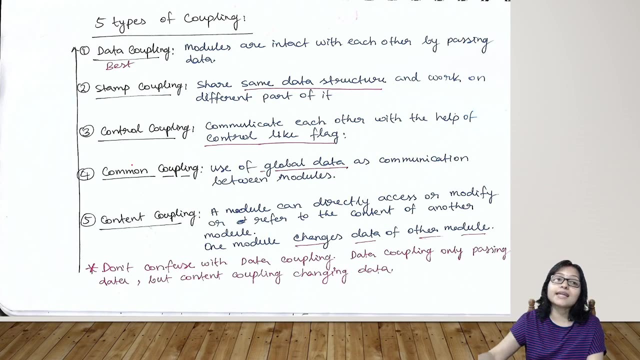 little bit easy tightness. so how much tightness is there? try to make it more easy for the necessary relationship. this is the target of the low coupling. we have to be low coupling, so low coupling. that's why the data coupling is the best one. data coupling why? because model 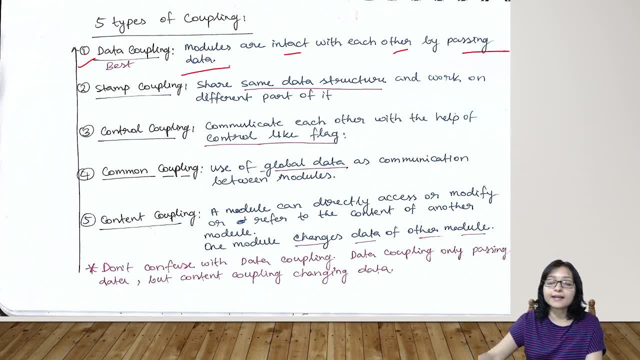 interact with each other by passing the data whenever some user is login. so after login, the user id will be passed to the profile only, nothing else. so it is a coupling data. coupling no relation. only I will pass the user id to the profile, nothing else. so it is good, one profile. 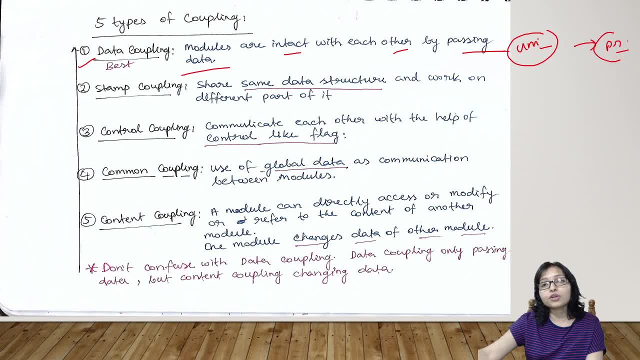 is a different module and login is a different module. so from the login module I am sending only the user id to the profile. so it is a good one. now no other relationship is there. stamp stamp means they are using the same data. 362 0030. 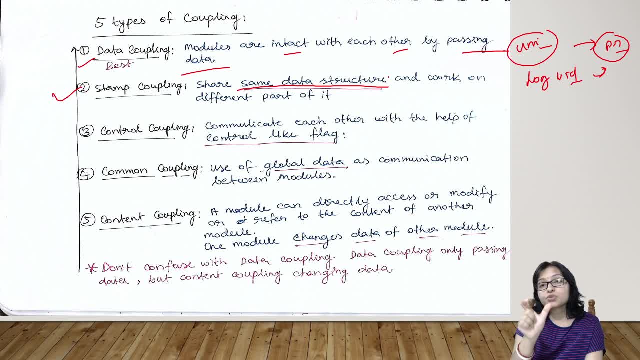 structure, maybe, and same array is utilized by when they are you creating a session. so when someone is used registering, then after that it is creating an array of session. maybe i am also using that same array. you are also using the same array. so model 1 and model 2 using the same array, same. 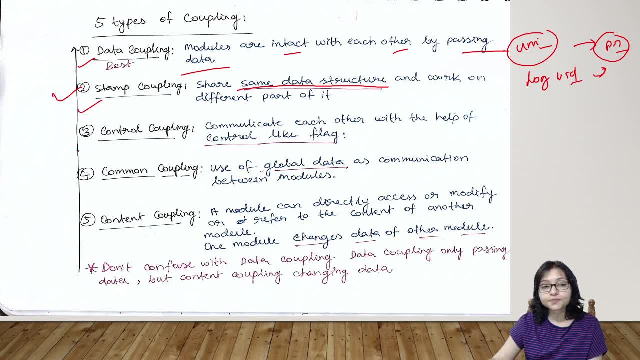 data structure that is called the stamp. next one is control coupling. control means same flag. there is some flag value i am also using like status. status is a facts, so my status is on or off. that is, using by two module. i am also using that same, another, also using that same, so status. 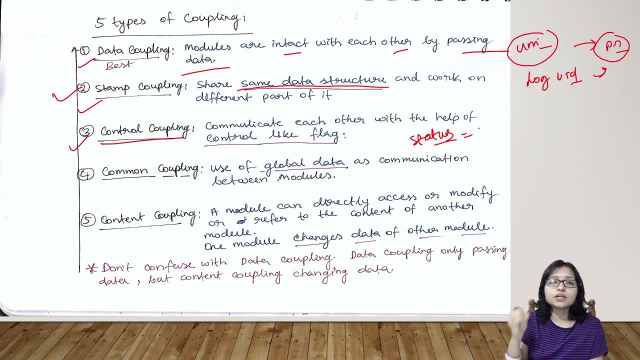 they are using. that is a flag, so it is a third one. that is control coupling. you are controlling with the same flag. next one is common coupling. common coupling means they are using the common ink global data. these are the main point, guys. that's why i have underlined the point, please remember. 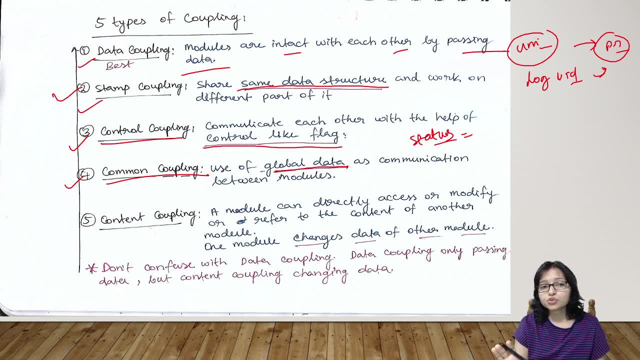 the main point and you can write down in your quick revision note. also, common coupling means they are using the global data content coupling. what is content coupling? content coupling means here. it is very bad and don't be confused with the data coupling and content coupling. data coupling is best one- it is passing only a data, but content is the worst one because 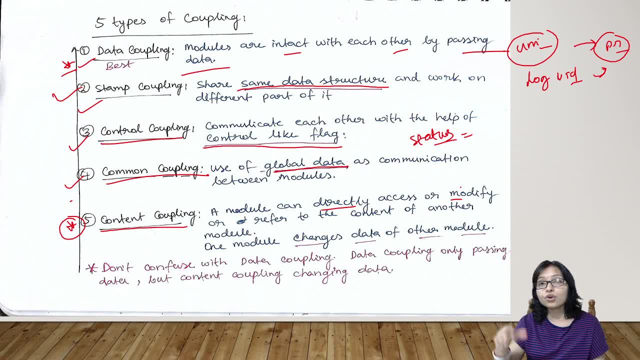 it is directly accessing the data. if your neighbor is coming to your home and he or she can access all your data in your home, it is not good. you are giving access to another one. that is not good. so if any other module can change your data, that is called the content, you are giving the access. 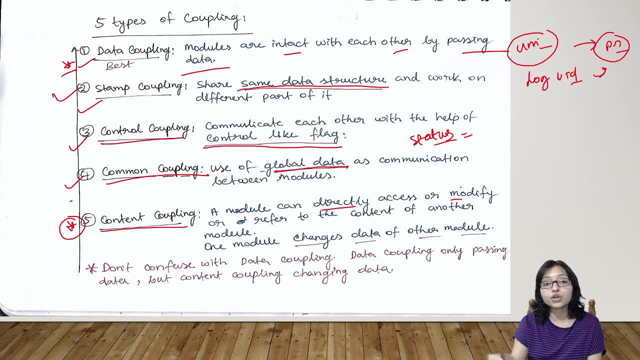 directly to your data and that is called the content. you are giving the access directly to another. one can access or modify your data. that is not at all good. that's why it is called the content coupling. so that's why i have written. also, don't be confused with the data coupling. 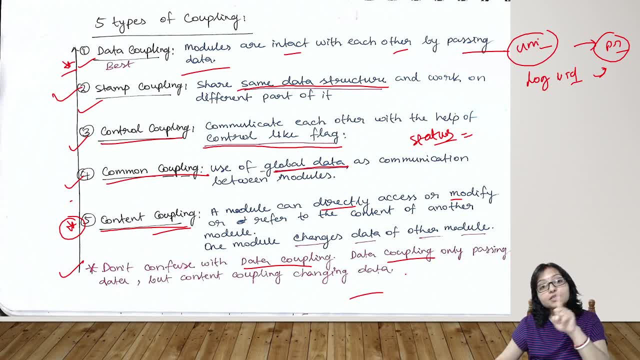 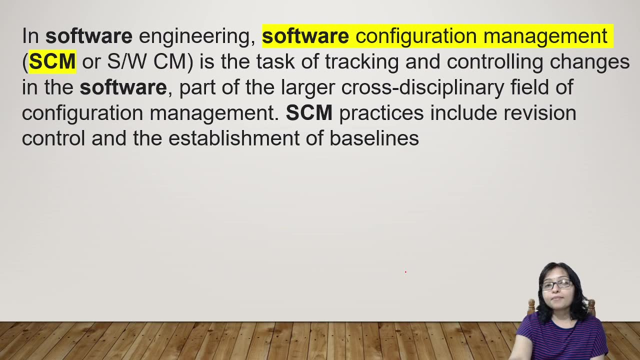 and content coupling. okay, data coupling is passing the data, but content coupling is doing that. it is referencing it right, it is changing your data. so now coupling is done. so calculation and coupling we have done. i hope still now you are watching. please write down in the comments so that i can understand. yes, 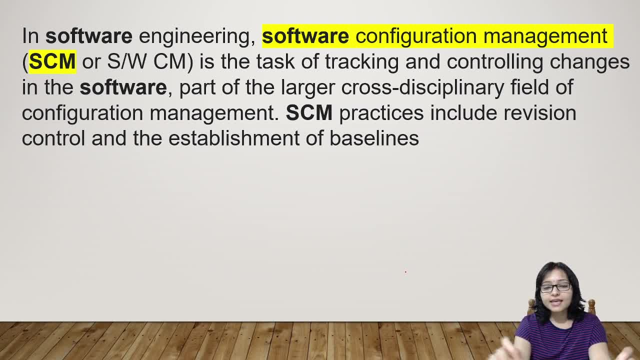 still now. i am watching. i am here in the scm we have done coupling and cohesion. please write down it will be good for me also for understanding. yes, students are watching. so now do that. key software engineering: scm, scm, how this scm is working. try to understand that. so scm means when we are doing a project, multiple team member is working right team member. 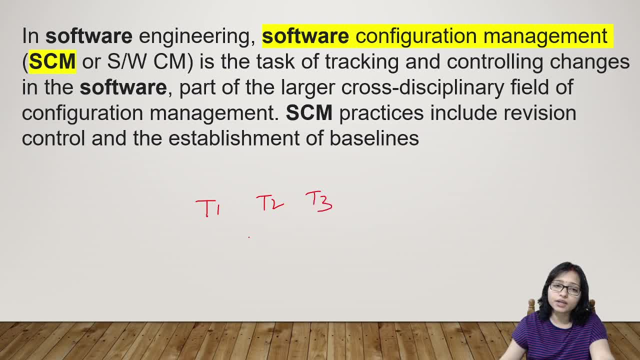 one team member two, team member three: everyone is working now always. it is a purpose that maybe i am also working in same page. you are also working in same page, now how we can work. that's why in the companies there are a global server means it is a company server and in that server all the updated codes are there and in our local machine. 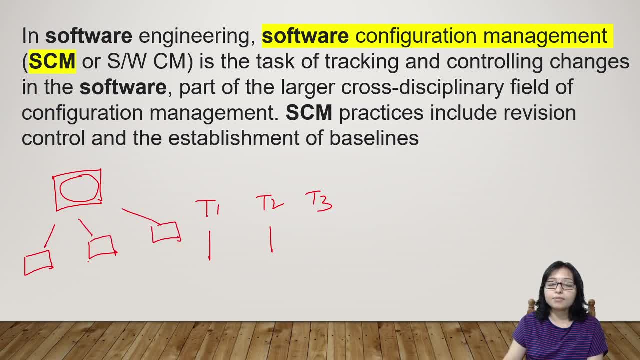 these are the all the local machine of each and every team member and in between there is the scm. in between there is the scm. what they are doing whenever they are coming to the company. they are coming to the office at morning. they will update the data. current final data. 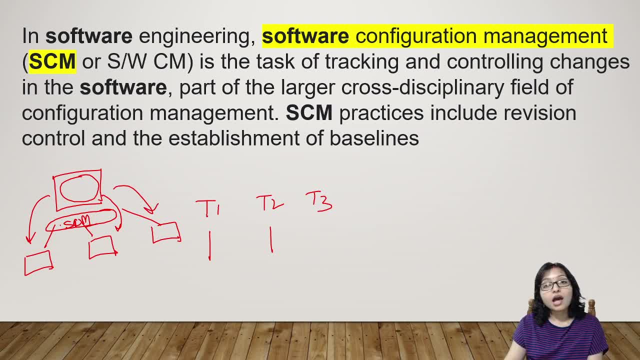 to their machine and they will do their work. after working their work, then they will again update it to the server before going to the home. now, maybe i was also working in a same page. you was also working in the same page. i want to update now. so i have updated my things. there was no problem. 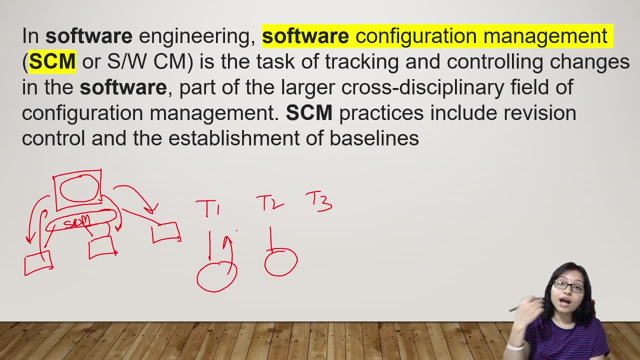 i went to my home. now, after 10 minute, you are trying to update it now. what will be the problem? as i have already updated, so if you will replace the page again, then my data will be lost, right? that's why, at the time of update, what you have to do whenever you have to update it. 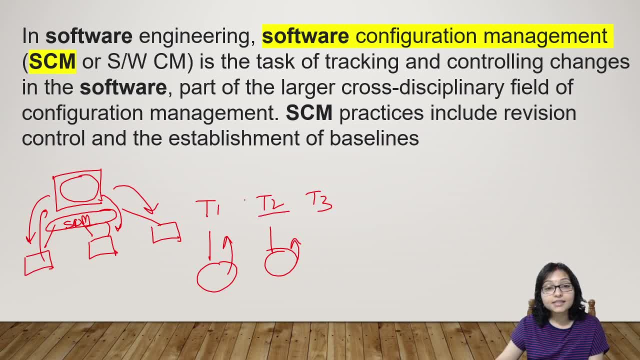 you have to check. the current version means maybe 10 minute ago, another one is updated, right, so you are checking the current version and the current version is check, showing you there are some new lines and there is maybe some conflict. whatever line may be, line number 52, you also work. 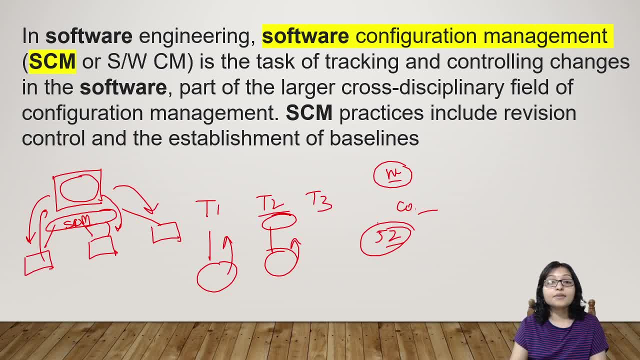 and i also work in line number 52, then manually, you have to check whatever i have done and whatever you have done, then you have to merge it together. after merging, ultimately your work will be not lost, my work will be not lost. then you will check the current version and the current version is checked. 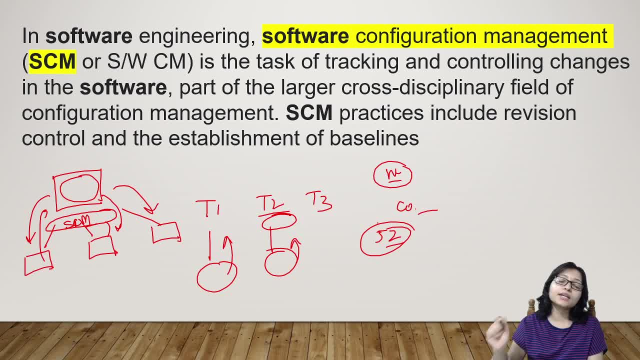 update it. that is called the scm, and scm is a technique mainly. example of scm is git, github. you all know parallely. all the person can work together, so version control is a big task of a scm and we are using the svn also. example of scm: okay, so now here there is version. 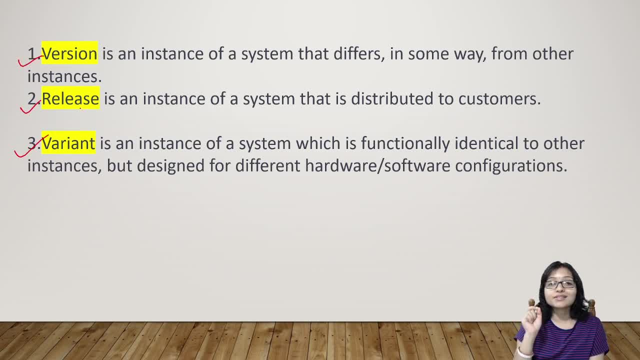 release and variant. what is version? what is release? what is variant? here it is actually maintaining by the scm. also, and this is very important, version means there is the different that maybe um one week ago something we have done and now we have done something. there is some differ, there is some changes. so instance: 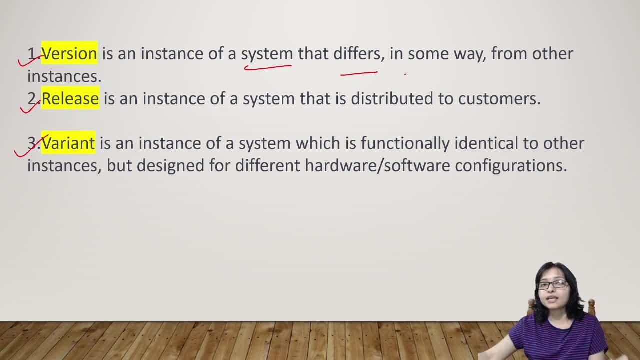 of the system differ some way. some changes are there. that's why it is called version 1.0. next one right release. what is release? release is that it is the instance, what is distributed to the customer. that is a release. and what is variant? variant means actually, functionality is same variant of. 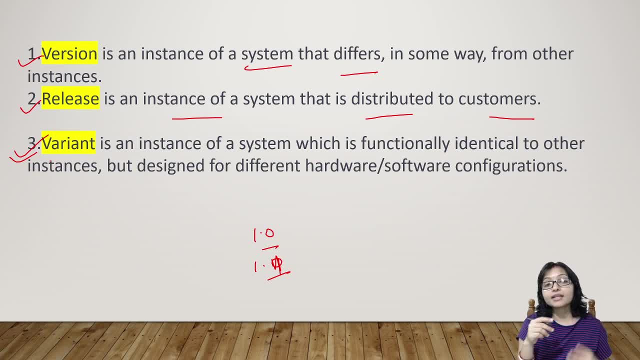 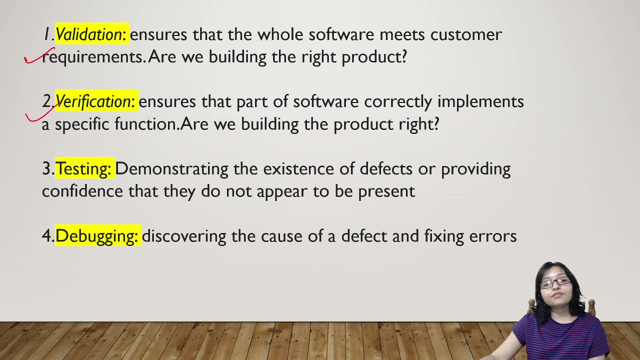 the car, then when the car is going to the, coming to the market, there are different, different variant. they are releasing, right? actual, these are the same model, same functionality, but some changes are there. that is the functionality. identification. are there right? so something includes such functions similar to the value protection. so again, within a 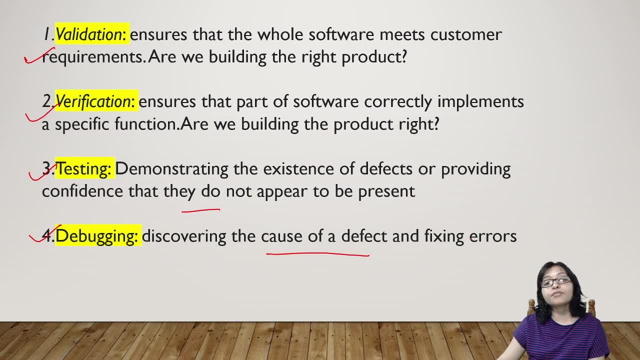 instance way is- i have tôur software. we are creating a cause of the defect and fixing it, and testing means demonstrating it and providing the confidence that there is no error. and what is validation and verification? it is very important. valley verification is the first one. then we are going to the validation. okay, so are we building a product? 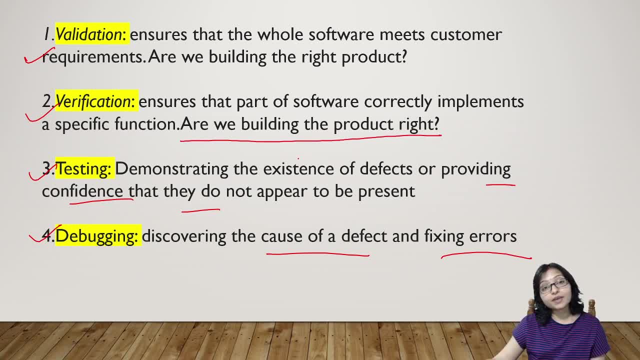 right means it is ensuring that whatever specification is there, are you doing the product, how the process you are following that process is okay, how you are writing the code. that process is okay means rightly, you are building the product. that is called the verification: you are very fine. the software implements specification. validation means: are we build the product right? 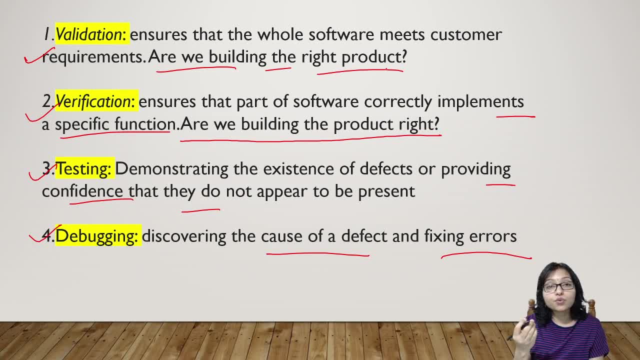 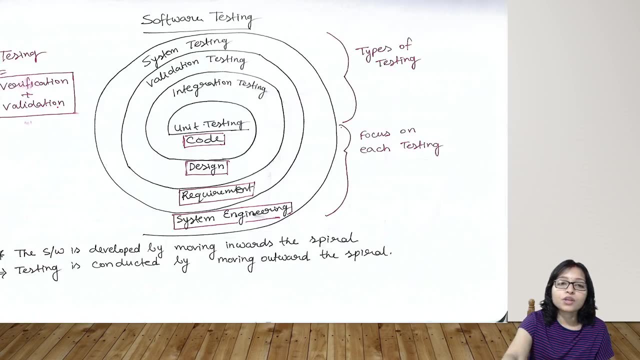 means right product. it is a correct one after building it is before, it is before. first we are doing verification, then we are doing validation. after doing the product, is it correct product? that is called the validation. so here now come to the point of testing. what are the testing testing? 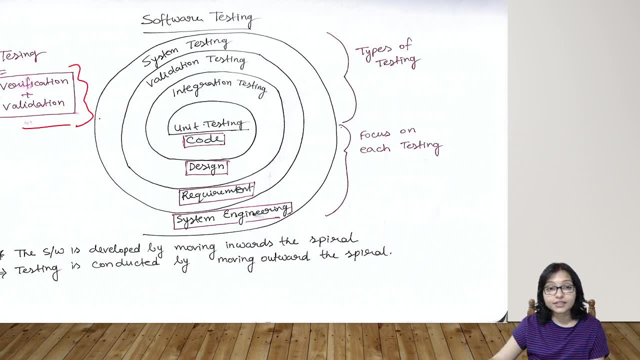 is the combination of verification and validation. so there are different types of testing: unit testing, integration testing, validation testing and system testing, and it it is. i have drawn in that way so that you can understand. unit testing is focus on the code, after that, integration testing is focus on the design, then validation testing is focus on the requirement. 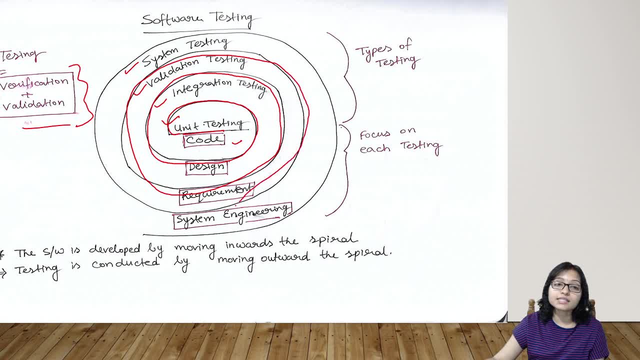 and system testing is focus on the system engineering. okay, so unit testing means small, small module. everyone is doing all the. i have done my module, then it is tested. that is unit testing. integration means when combining all the modules- three to four module, five module done, now they are combining all the module. after combining all the module again, it is 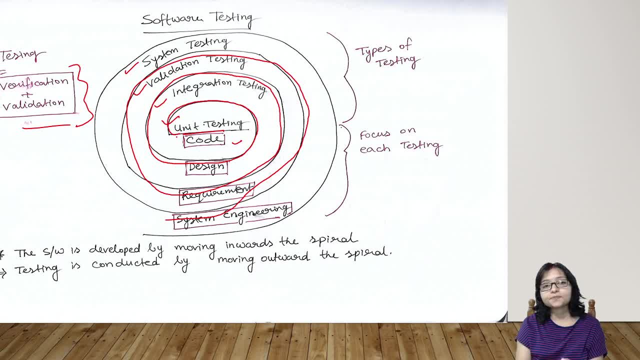 tested. that is called the integration testing. and now the total project is done, total product is done, then you are going to validate it. that is called the validation. the product is right. customer asks you to make a bicycle. is it a bicycle or it is a scooter, or you have done a bike. that is the validation. and finally, 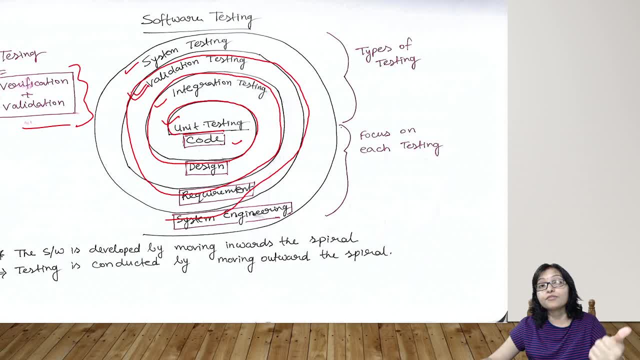 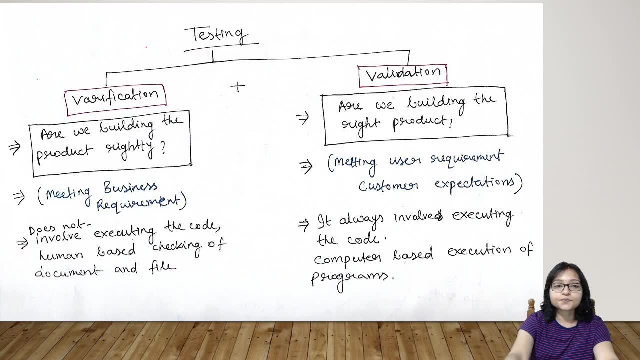 your product is tested. now you are uploading into the environment system, the server. now it is working fine. that is called the system testing. so here i have written also the verification and validation. so are we building the product rightly? and here are we building the right product. it is meeting the 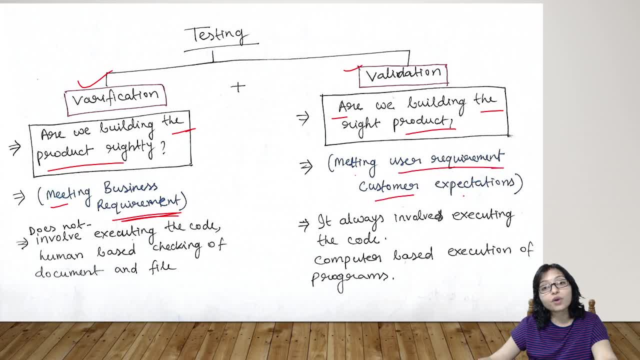 business requirement and it is meeting the user requirement of the customer expectation does not involve executing code. human based checking is there for the document and file and here always executing the code because ultimately you are checking all the purpose is correct or not. that is always it is doing. 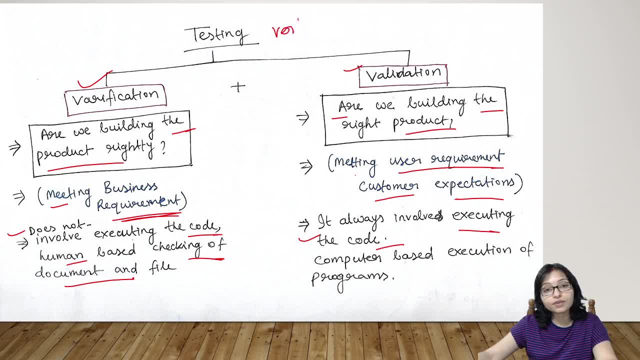 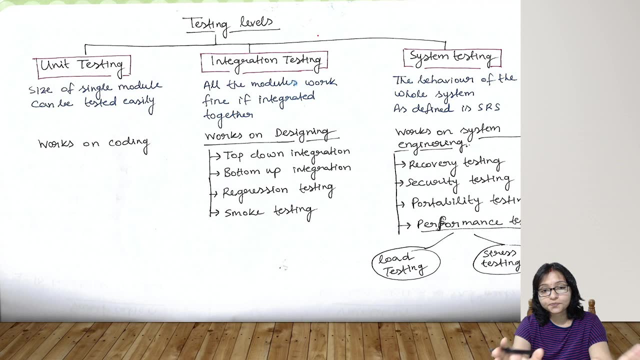 and always remember verification. first we are doing verification, then we are doing validation- verification when you are doing your work. at that time you are checking validation after product is done. that is called the validation. now come to the different types of testing level. it is a quick revision chart for you. 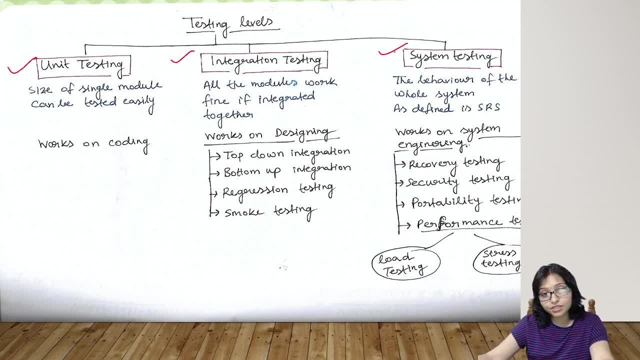 you need testing: integration testing and the system testing. so unit testing is already. i have done integration testing also. i told system testing also. i told here these are the part of different, different testing: top down, bottom up regression and smooth testing is under integration testing, under system testing. there is recovery, system security, portability, performance and under 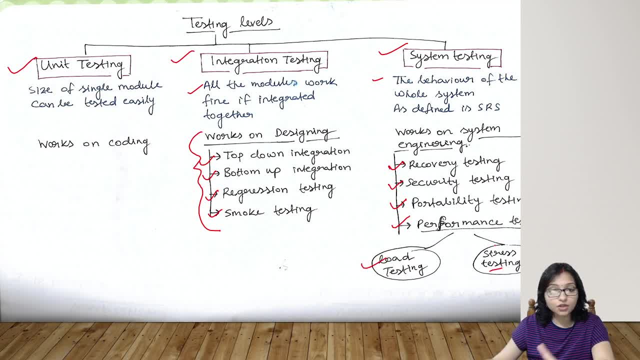 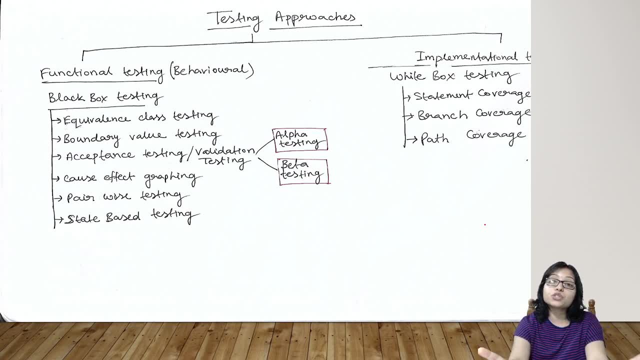 performance. there are load testing and stress testing also, so this is a quick revision chart for you now. uh, testing approaches are dividing into two way. one is functional testing, another is implementational. functional means behavioral testing. that is called black box testing. under black box testing, there is equivalence, class partitioning, boundary value analysis, acceptance. 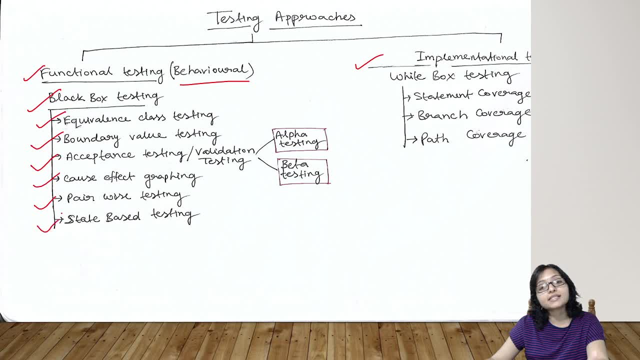 testing, cause and effect testing, pairwise analysis and state-based testing. white box: statement coverage, branch coverage and path coverage. and already the videos is there for the statement coverage, branch coverage, path coverage. i am giving the link in the top. you can see in the i button. must watch that. it is very important, part and other than that. 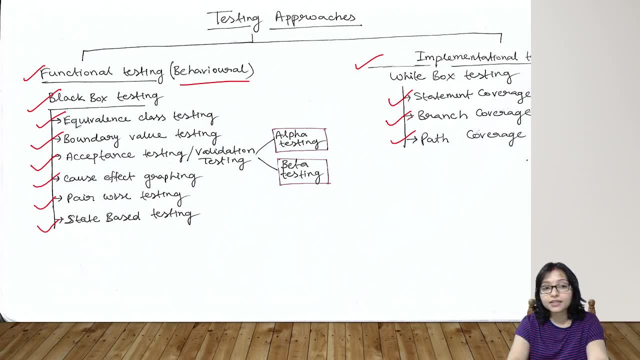 the software engineering playlist is also there. you can watch the playlist also and after that also, if you are facing any issue. if you want some videos from me, then definitely let me know. and what is alpha testing and beta testing? alpha testing means it is inside the organization before releasing to the market. when it is checking inside the organization, 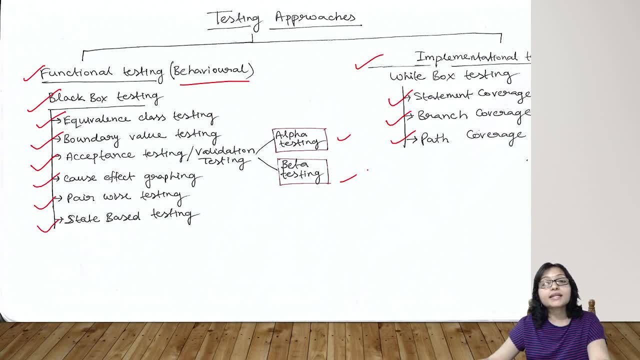 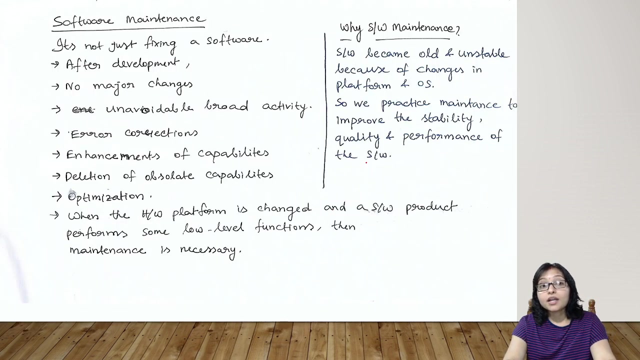 that is called the alpha testing. and beta testing means it is released for a limited number of customer and the customer is checking the version and after that they are providing the feedback. it is called the beta version means real time environment. the testing is going, it is by the user. that is called the beta testing. now come to the software maintenance. so we are 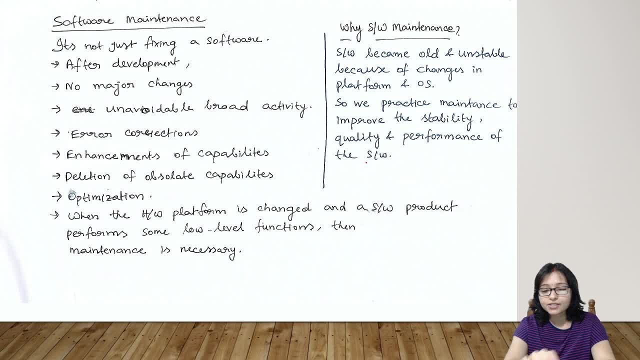 coming to the next part, that is, software maintenance. so please write in the comment section. yes, ma'am, till now i am watching and now we are doing software maintenance. we have done the software testing. so, in detail, if you want to learn the software testing, then let me know in the comment section so that i will upload a specific. 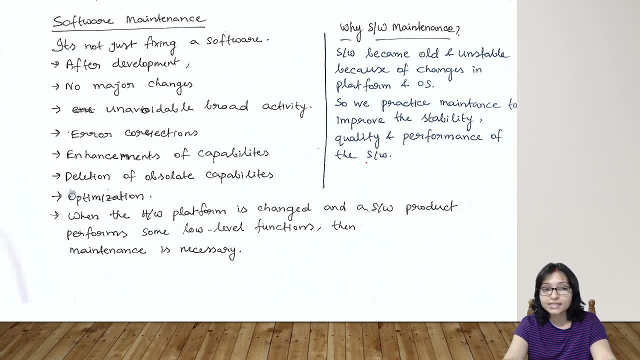 video for software testing, only different types of testing. now see here the maintenance. what is maintenance? what is the main target of the maintenance? just, it's not just fixing a software here after development. no major changes is allowed here. unavoidable broad activity means there are some. what is i cannot avoid. we have to maintain it. there is water is not. 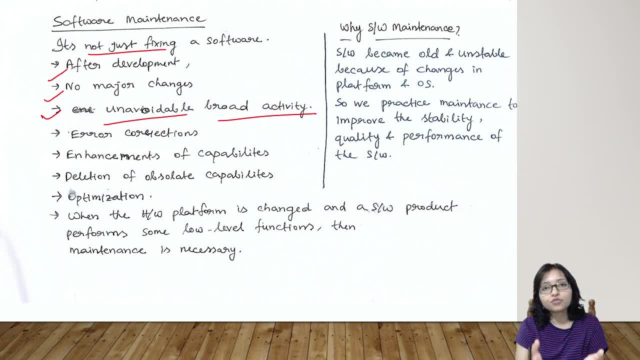 to your home so you have to call the plumber and you have to fix it. that is unavoidable situation, right? so some unavoidable situation can be there that you have to control for the maintenance error detection. some small error can be there that you can do, detect and correct it enhance. 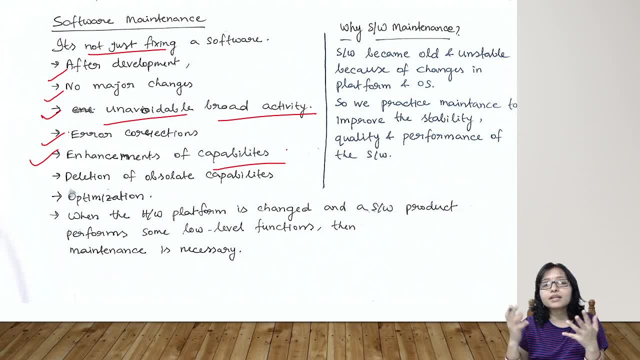 of capabilities. they are. your capability means hundred user are coming, then working is fine. when the thousand user is coming, then it is not working fine. so capability also have to be deletion of obsolete capabilities. what capabilities are not working now? it is not required that we can delete. and optimizing means time, more optimized query: you have to write so. 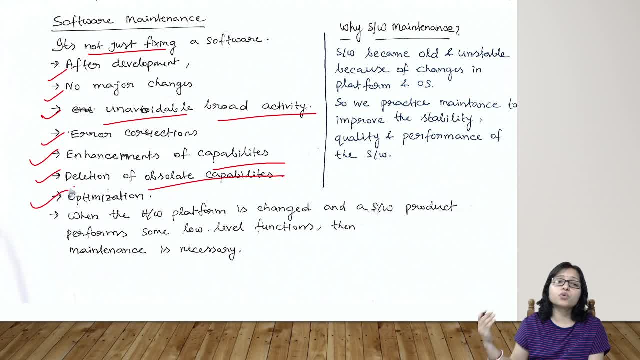 that it is taking more time. maybe when the load is more, stress is more than it is taking more time, so we have to optimize it. this is that the main purpose of the maintenance. and what is maintenance? that become old and unstable because of changes in the platform. 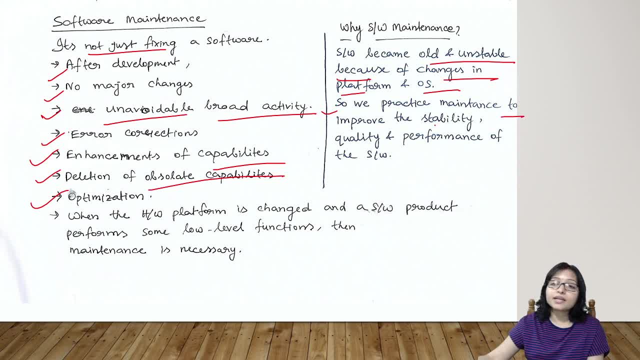 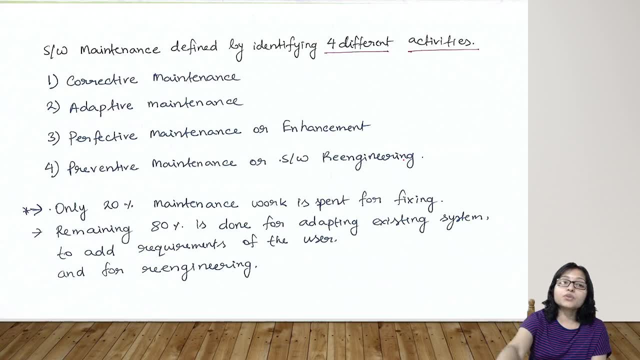 or operating system. then we practice the maintenance to improve the stability and quality of the performance. that is all software maintenance. now there are different types of maintenance and these are very important question are coming from here: corrective maintenance, adaptive maintenance, perfective maintenance and preventive maintaining. Corrective maintenance means what? 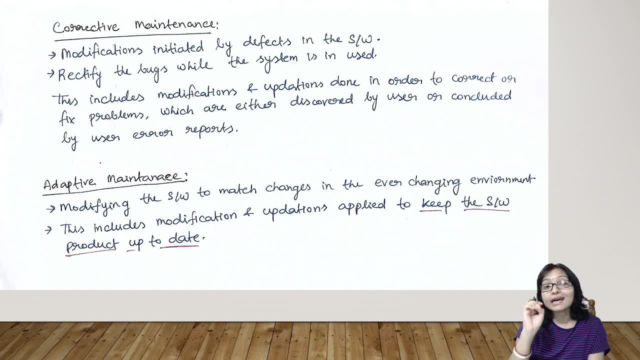 Corrective maintenance means we are doing only correction defect initiated by the defect. Here is some defect like bug fixing you are doing. that is called the corrective maintenance means fixing defect. corrective. Adaptive means new platform. Remember that adaptive means ever changing environment. 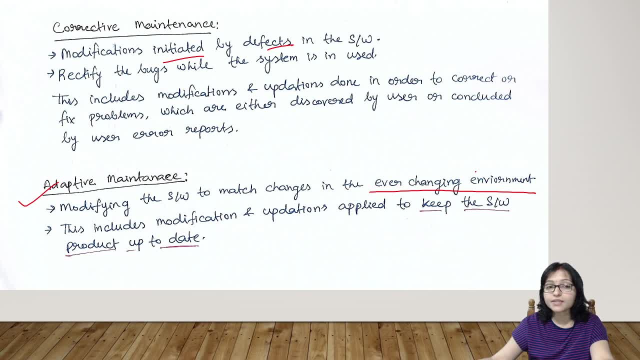 It is related to the new platform, new environment- that is called the adaptive maintenance- and keep software up to date. This is the main purpose and the keyword of adaptive maintenance is new platform or new environment. Remember that Next one is perfective. Here, most of the time, student are getting confused with perfective and adaptive. 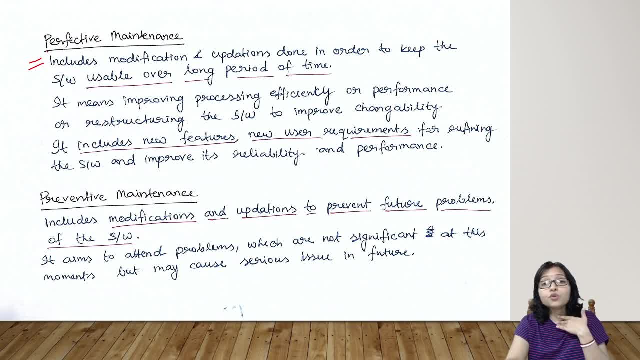 Perfective means here: I want to be more perfect. That's why I am trying to add some new feature. I am trying to do record my video in different, different ways so that you will be more happy to watch that video, Right? So it is called the perfective. 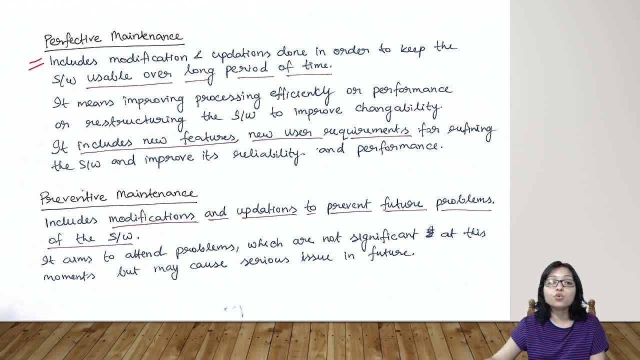 Day by day, improving ourselves by including new feature, By including new feature or the new user requirement. I am asking you what type of video you want from me. That is a new user requirement And new feature. that is called the perfective, So usable over the long period of time. 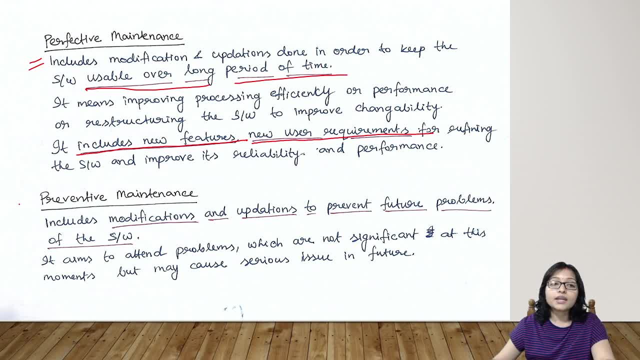 That's why we are going for the perfective maintenance. Next one is preventive. Preventive means in future, maybe some problem can be happen. That's why now we are taking the precaution That is. prevention is better than cure. So that is the prevention. 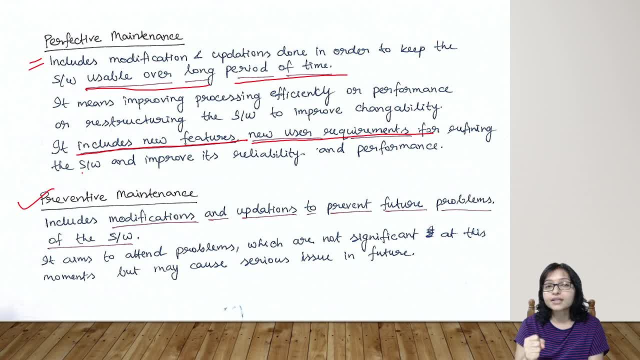 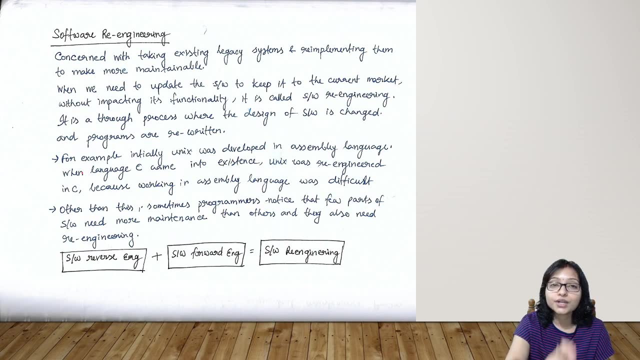 Nowadays we are taking more prevention so that we can protect ourselves. Same thing when you are doing for the software. that is called the preventive maintenance. So now all four types of maintenance is done. Write down in the comment. Yes, Maintenance is also done. 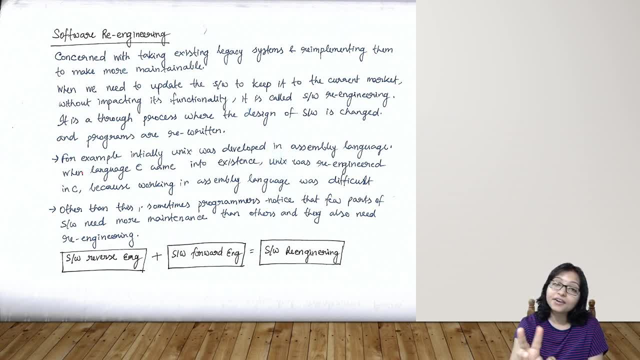 Now come to the software: reengineering and reverse engineering. What is reengineering, What is reverse engineering? Why we are doing the reengineering Notes is already there. You can go through it. Just I am telling you what is there. Reengineering means that when it is a old project, legacy system means legacy system means it is a old project. 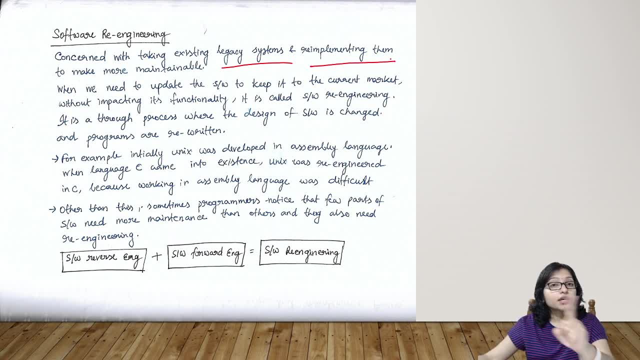 Now you are trying to re implementing it. It is not a new project. Remember that it is not the new project. No new functionalities are there. Maybe you have built a software previously in C. Now you want to change it in Java. Then we are doing the reengineering. 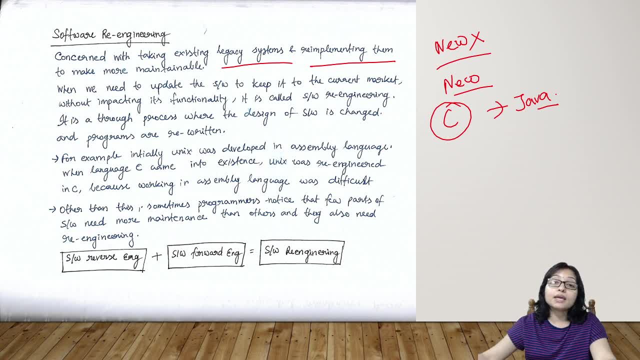 engineering. now the problem is there. maybe five years ago you have done the project in c. now, after five years, you want to do it in java. now client is telling you: i want to do it in java. client don't have any documentation, any requirement, any design in their hand. now the problem is that 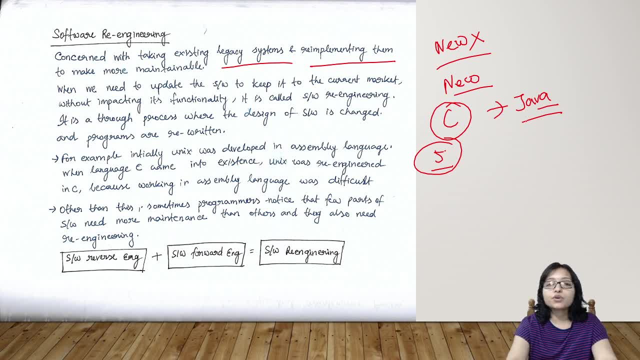 how you can do. they are telling: it is my project, i want to rebuild it, i want to re-implement it. so what you have to do? that's why we have to do the reverse engineering. re-engineering means reverse engineering plus forward engineering. why we are doing reverse engineering, reverse 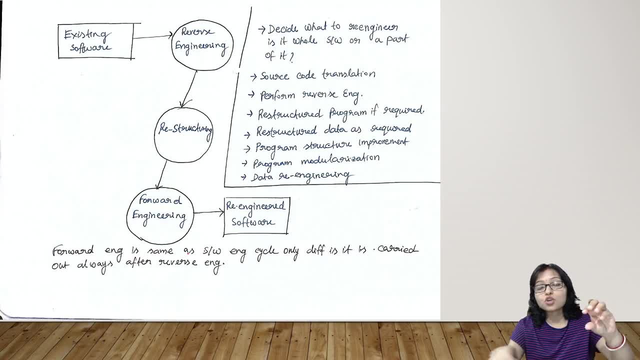 engineering is that keep detecting from the existing software. you have only the existing software. you don't know anything. so for a time, maybe for five days or ten days, you will only visit the software. you will try to understand the software. what is going on you? so, uh, that is called the reverse engineering, that is deciding what the re-engineering source code. 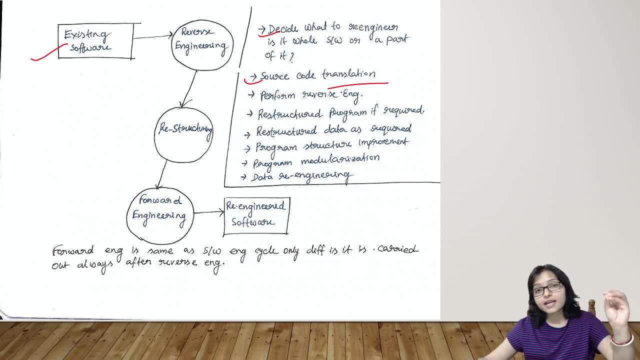 translation or everything means you are trying to understand so from the old project, from the existing software. now you are trying to understand the design of the software, requirement of the software. that's why it is called the reverse engineering. normal engineering was: first we are doing requirement, then design, then development, then compliance, then design, then development, then. 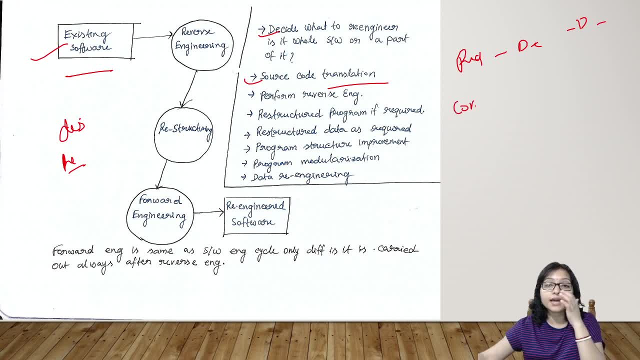 complete product. now you are doing from a complete product. you are trying to understand the design, you are trying to understand the planning and requirement. that's why it is called reverse. you are going in reverse direction direction. that's why it is called reverse engineering. so, after doing the reverse engineering, now you know the requirement, now you know the design, now you can. 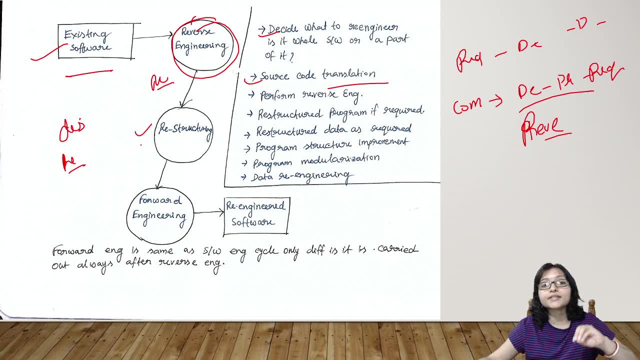 restructure it. now you can do the code, restructure it. then you will do the forward engineering. you will write the code and everything. then you will deliver it, the re-engineered product, to the customer. it is called the software re-engineering, and that's why re-engineering is reverse engineering. 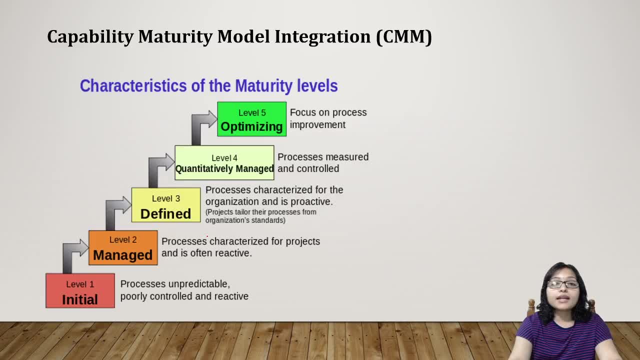 plus forward engineering. now, finally, this is the last slide of this class and i hope that you have till now you are watching- and last one is cmm. level of this is nothing else. these are the companies level. company's level means like cmm level one, two, three. 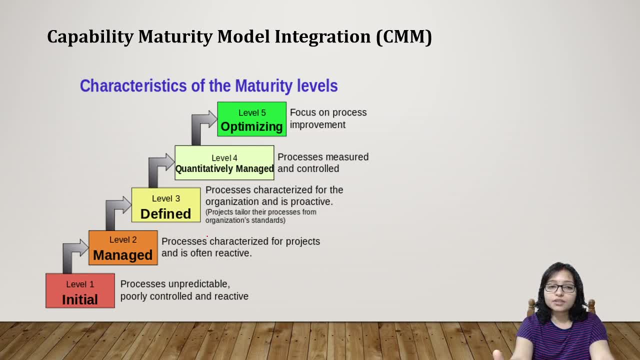 four, five. don't cram it. no need to cram it. what is that initial R means new companies. what are the currently just startup companies that are called the initial? so when they're startup companies, they're not thinking about anything, they're just trying to understand what are going on in the 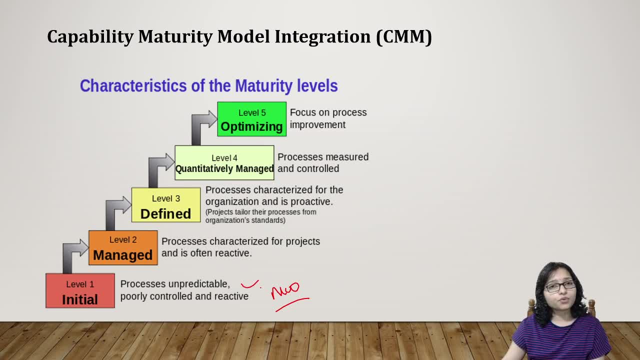 market. so process is unpredictable. you cannot predict the process. and poorly controlled it is not not that much control because they are new companies. managed now the level two. managed means it is categorize the project, this, this type of project. it is focusing on the project more because 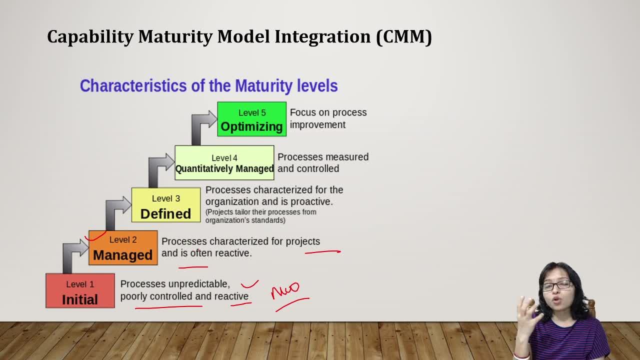 if i can do a project properly, then i can do this type of same type of project multiple time. that's why it is focusing on the project management more. level three: in the next level it is called the defined. now they are focusing on the process definition, process character. 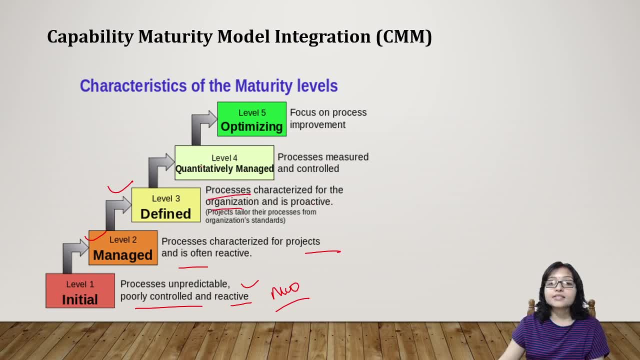 understanding, and then they are focusing on the process, definition, process characterizing, that is for the defined. next one is level four. that is qualitative managed. okay, so level four is here. now process is also. their quality is also there. that is level four. level five is optimized. now level five companies are totally optimized. they are focusing on the project, quality also. 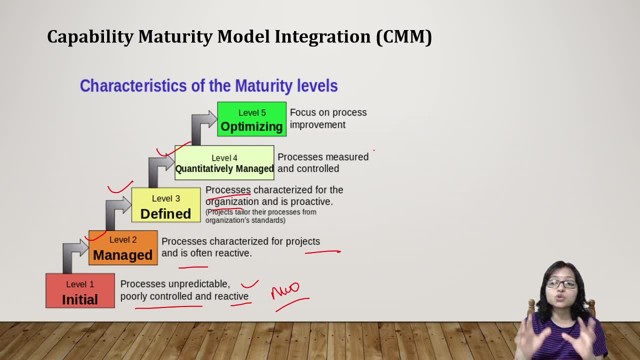 process quality also, team quality also. they are focusing on the process quality also, team quality, also how the project is going on, if each and everything they are thinking about that, because they are now the higher level company, that is called the level five companies and this is all. 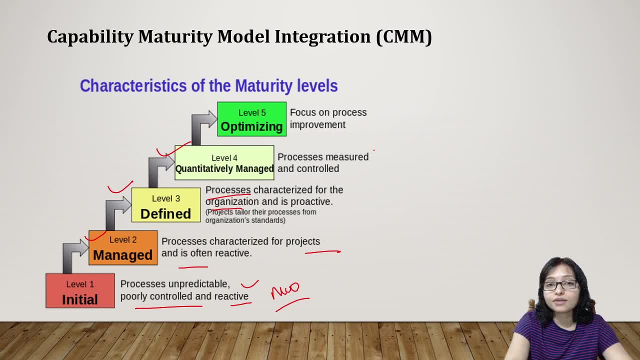 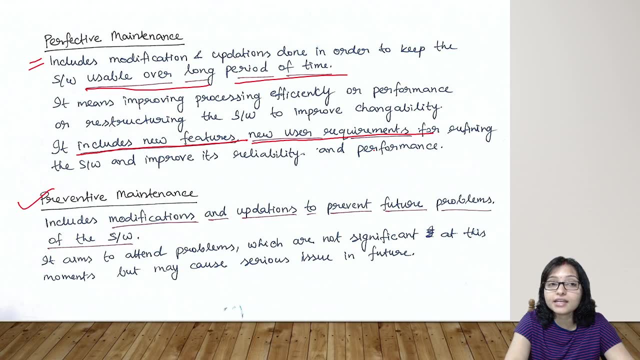 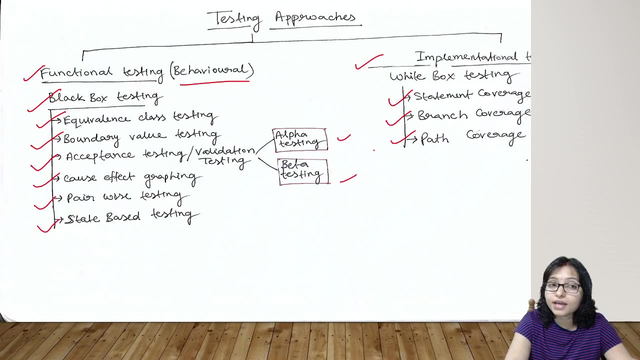 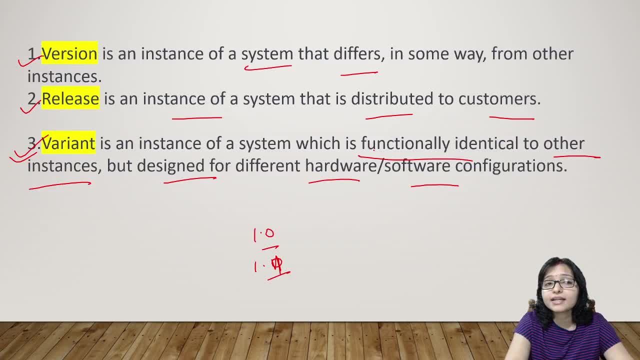 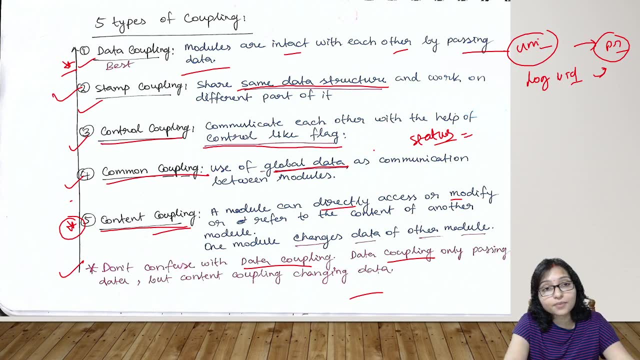 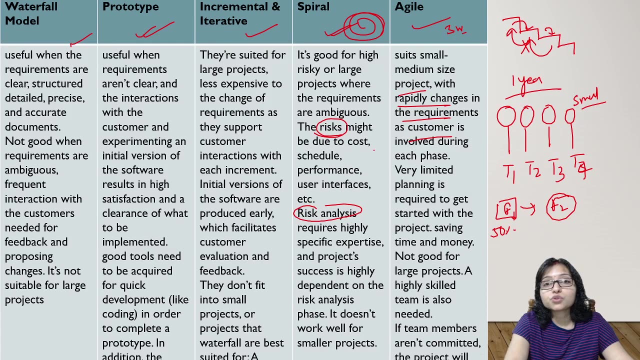 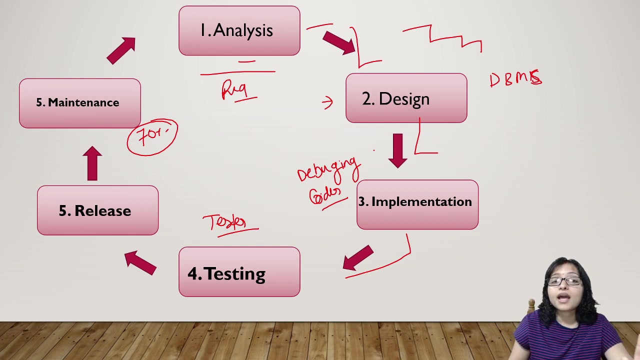 done. what is the difference between debugging, testing, verification, validation, what is version release, variant, what is SCM? different types of coupling, different types of cohesion, and after that we have done different types of software model also. so these are the very important area of the software engineering from where always question are coming, and after watching this, 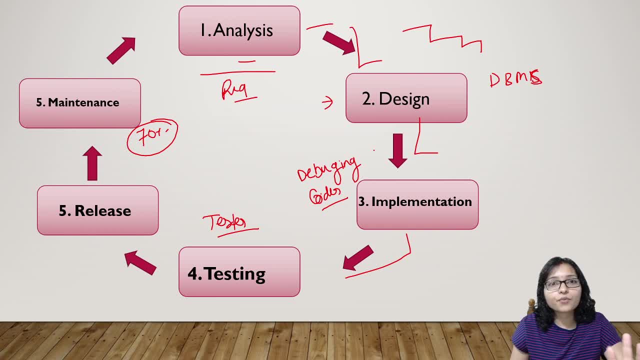 video. i hope definitely you will get some question from this. it is hundred percent confirmed. definitely question will be there from this video and please, after atteming the exam, definitely let me know in the comment section how many question was there and how many question you are able to. 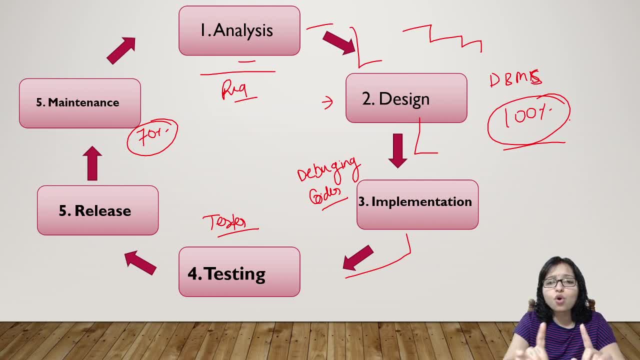 do properly from this video, because in this video all the important topic, theoretical topics are there in this video. so if you are interested then i will upload the numericals also. i will upload the uml also, but it is depending on your interest and for that share more and more you have to share the video as much as possible so that maximum level of views. 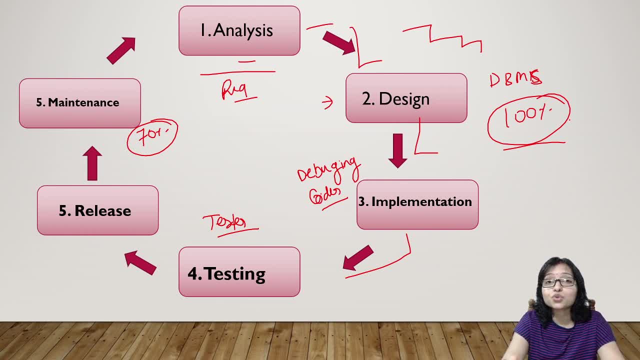 maximum level of likes and comment i can get so that i can be also get some motivation. then i will upload more videos in other subject also and more videos on software engineering also. thanks for watching this video till the end. definitely share this video and stay tuned with this channel for more videos. thank you, bye, bye. see you soon in my next video.